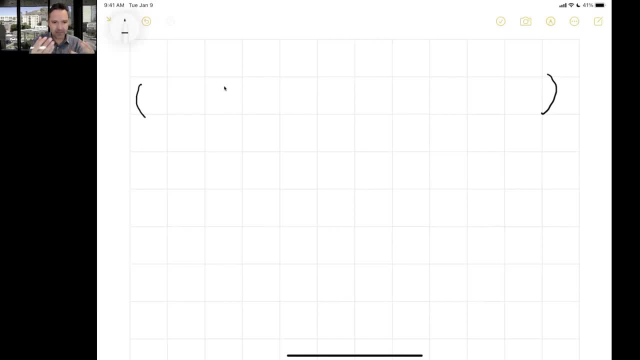 word. after you open the parentheses, the instruction that you want to execute is going to be if more over. remember this is not case sensitive. you can use if, or you can use if, or any combination. open parenthesis, closing parenthesis. the first part the instruction. second white space. and what is the other thing that we need in an if condition, and it usually after: 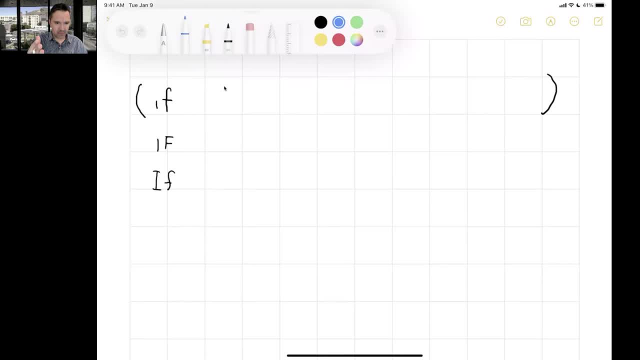 the keyword if, the condition. the condition is going to be inside of parenthesis, not because the parentheses are needed as part of the syntaxes of the if, but because that one is a call to a function, for instance from here. so to explain in little more detail, sort any predicate. if you remember, that is the particular name for those functions. 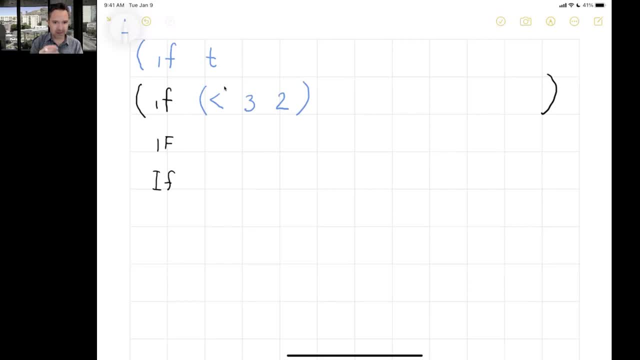 Function. if first parameter is the condition, Next, what do we need? Usually, if you have an if condition, you have two possibilities: Condition true, condition false. If the condition is true, you execute something. If the condition is false. 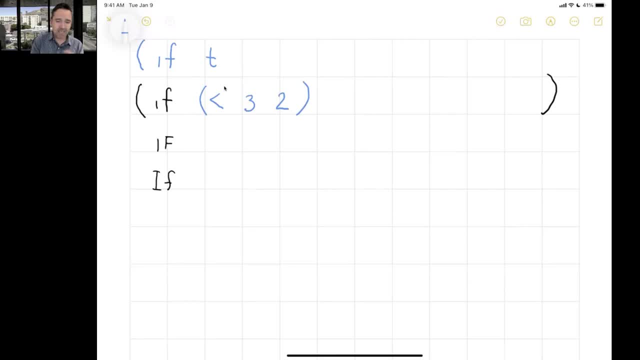 you do something else. Similar idea: Open parenthesis, closing parenthesis. Whatever I put there is going to be executed only if the condition is true. Optional. I can put another one, And that one is going to run only if the condition is false. You can have: 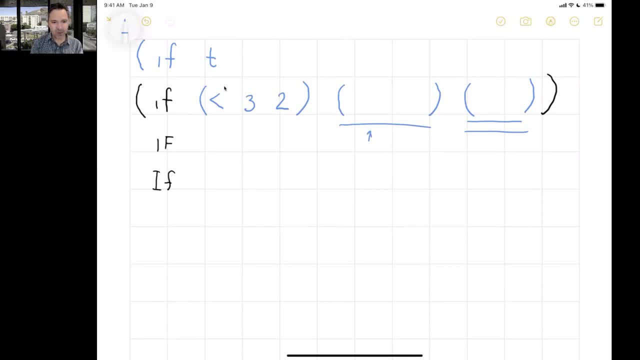 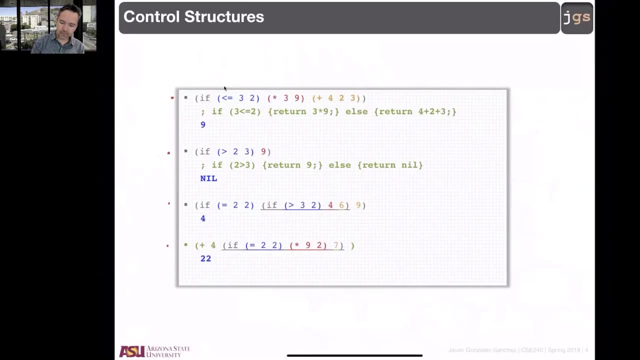 only one, Like an if, without an else, Or you can have both. This is the syntax for an if condition. here Examples The first one. I am giving you the instruction in Lisp and in a comment the equivalent in other languages. Useful reference: If in blue the condition: The condition 3: lower or equal than 2.. 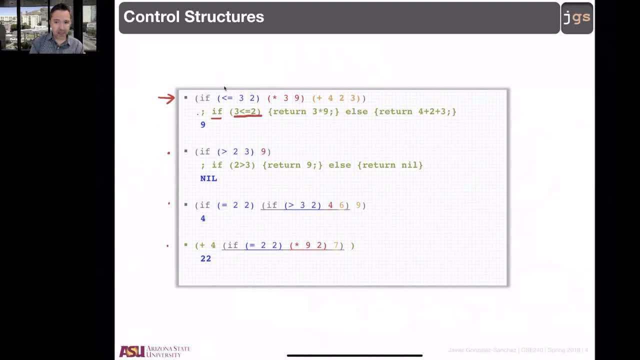 If the condition, And then red And orange. If the condition is true, execute the instruction in red. If the condition is false, the instruction in orange. In this case, three lower or equal than two Condition false. If the condition false. 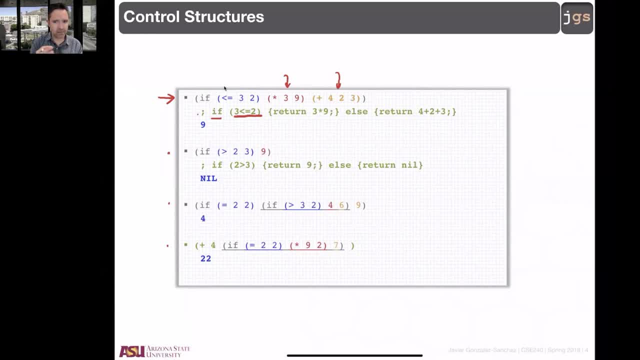 then execute the addition of four, two, three Format data: The if, like any other instruction in Lisp, returns a result. When you execute the if, you are going to get a result. What is going to be the result of the if? 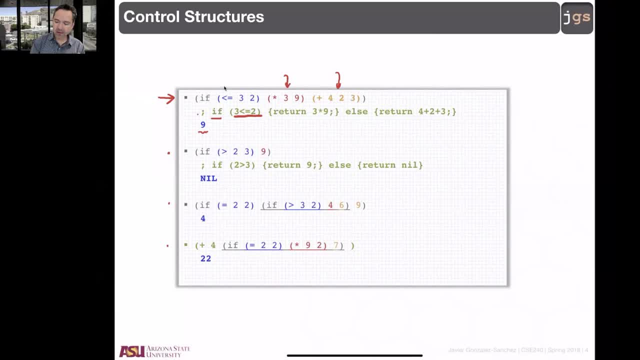 The result of the statement that is being executed. So this instruction, The condition, is false. I am not going to execute the red one, I am going to execute the orange one. The orange is going to do the addition 4, plus 2, plus 3.. 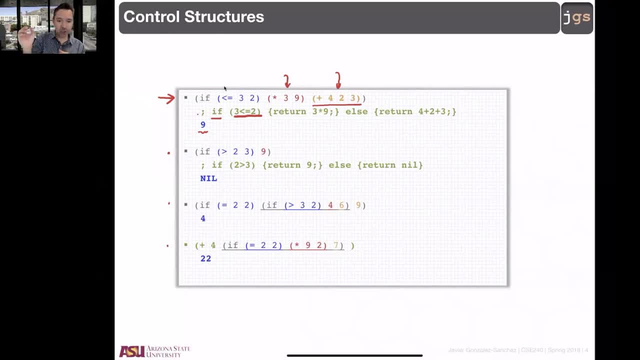 That is a function that returns a result. It is going to return the result, this plus to the, if Just like that. It is a function inside of a function And this one is going to print. Everything is a function. Everything returns something. 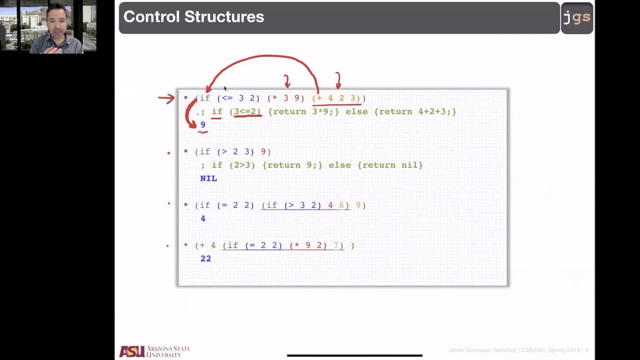 Even the control structures, Even the if. So in this case, if you copy paste that line, you get the 9.. And that line is telling you that this one executed because this condition was false. in this case, That is an if. 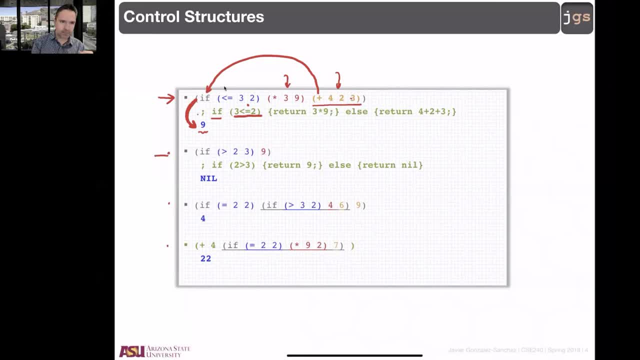 Second example, Exactly Following with the question in the chat, This is like condition, question mark, operator action, colon action, But instead of the question mark, the if at the beginning And the colon. We do not need the colon. 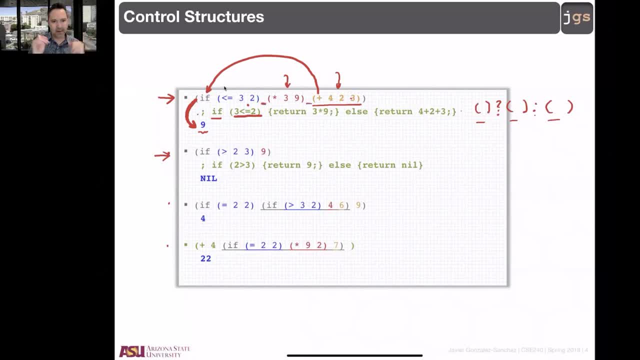 We use white spaces and parentheses. That is it. Second one In the second one is an if without an else. And let me be clear Here in Lisp: always, always, always. a function returns something, Always There is no void. 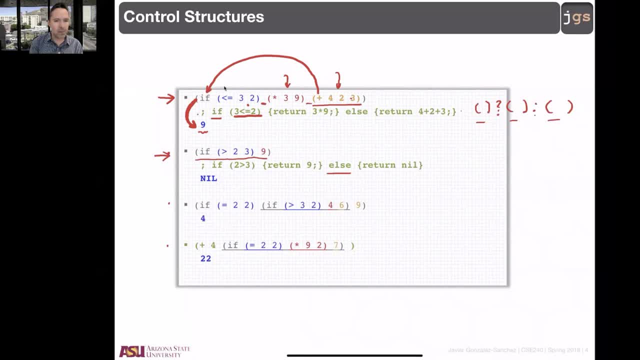 So in this example, If we think about that one being an if without an else, The big question is: well, what is going to happen when the condition is false, Just like in this example? The condition is false, I am not going to execute the instruction in red. 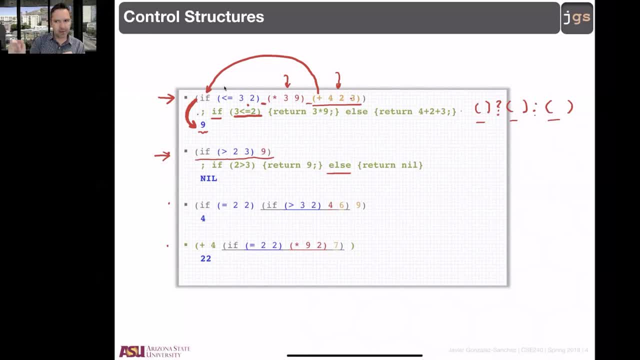 That is the second one, But I do not have another one. Well, if you do not have another one, that is your result. Nil, I do not have nothing to do. I do not have a result. If you think about the translation of this instruction to another language, what we are doing is something like this: 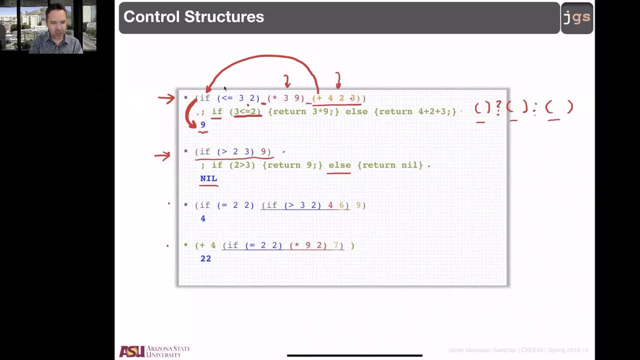 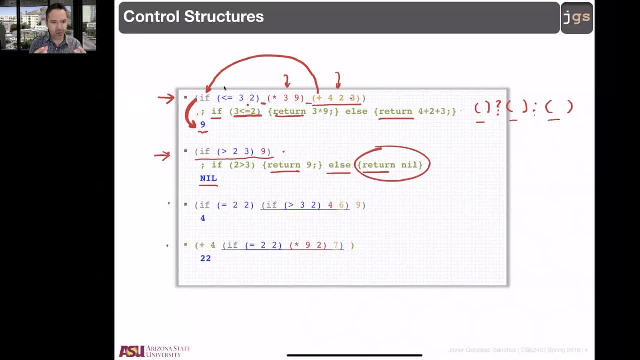 You have a return. A return is nil or null, Always. Now here You have a nine, without parenthesis. Yeah, What happens if I want to return the nine? I do not need to force an operation like plus five four. 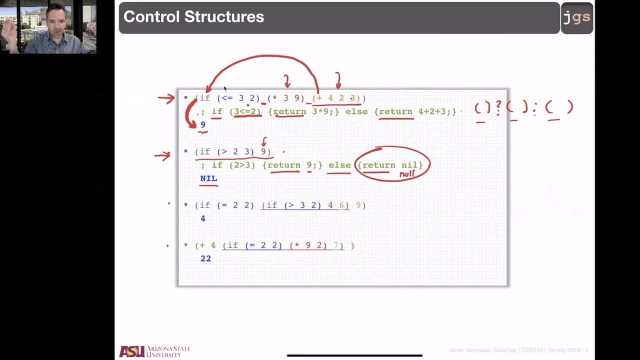 If I want to return the 9,, if I am sure that is the 9 that I want to return, I just put the number. Remember, the parameters can be an atomic value or a function, always, So you can have a combination. You can have something like open parenthesis if t 5, 4.. 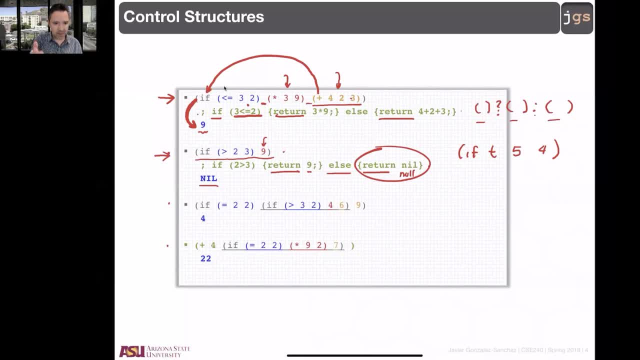 That is a condition That is correct. If is the macro, the function and the parameters, the three parameters that I need, The condition, what to do when the condition is true? what to do when the condition is false? The condition- an atomic value- true. So it's like if. 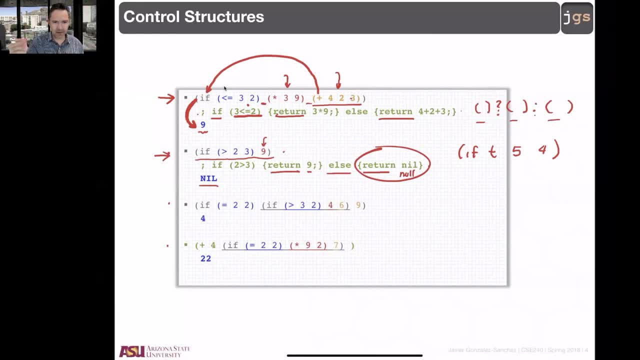 parenthesis: true in Java, Always true. It's not really useful, but it's correct in terms of the syntaxes. Okay, it's true. What is going to happen? We're going to return the 5.. Just like in this example When we're going to return the 4? Never, If true, return 5.. Else. 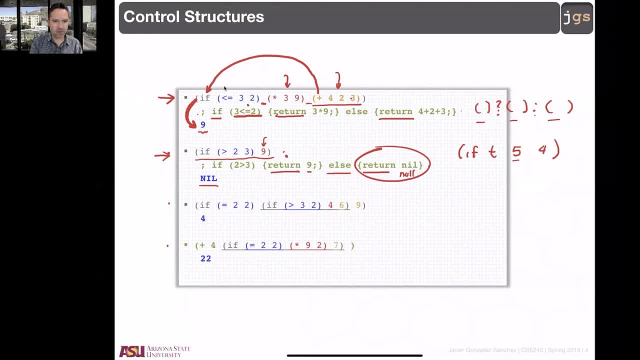 return 4.. The condition is always true. The return false is never going to run Again. do not make a lot of sense, but syntactically it's correct. It's an instruction in Lisp and can be translated to other languages. So atomic values without parentheses. The parentheses are because 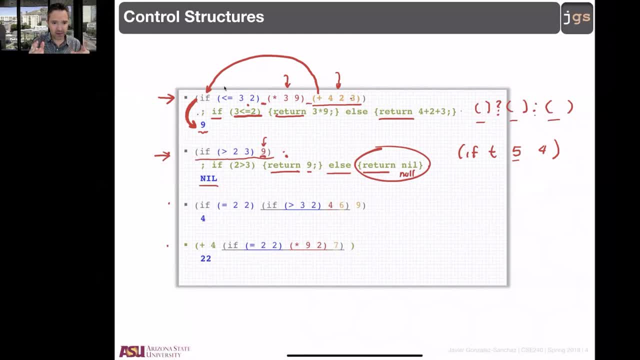 another function is being called. Just remember that one. So another one. We can make things a little bit complex, Like: can I put ifs inside of ifs And I didn't put here the equivalent in another language. but we can do it. 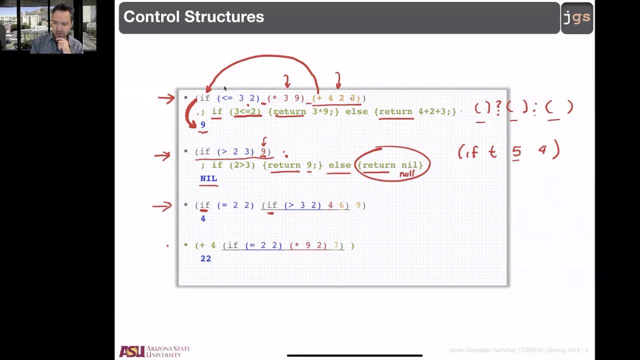 It's like you are telling me here that you have an if condition, that the condition here in blue is 2, equal, equal, 2.. Hopefully you remember the equal equal. in Lisp is used: one equal. We need to review what to do with the signature. 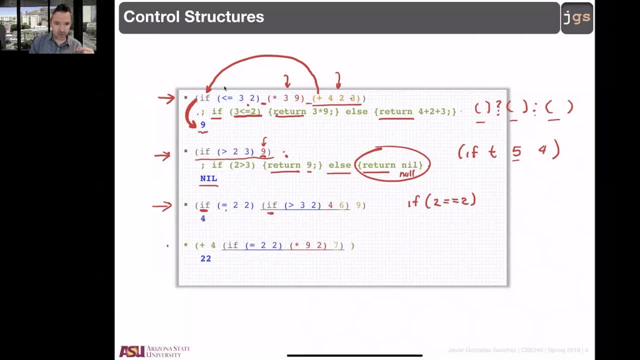 But this guy is this one: C, C++ on Java. So if that condition, something, that something here is starting here. all of this until there. Did you notice the gray parentheses? and inside we have another things, The only thing that's. 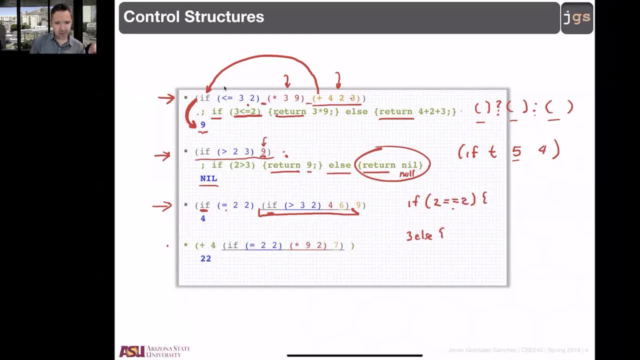 I know is on the Ls part. the last thing is a nine. The nine. this one is going to be returned if this condition in blue is false. But if that condition is true, what I have as a second parameter is another instruction. if in parentheses, That is the same as having here. 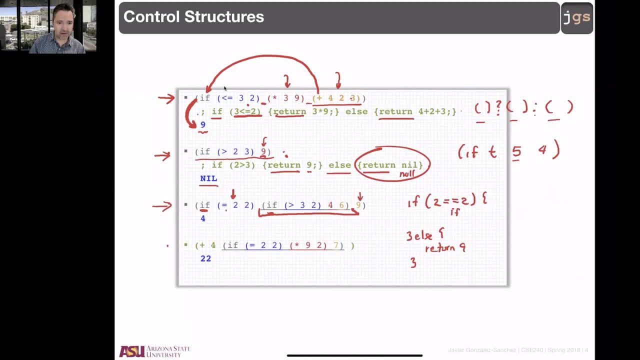 a planes, an underscore, an integer, an integer, an yes, an integer, an integer. here, another if with its own condition and its own body. for this new if, the condition is another function greater than that is equivalent to this. this in blue is the condition of the if that is inside of the other if. 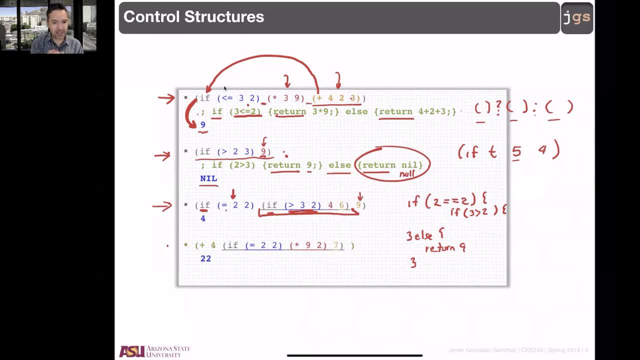 and notice that here, when we talk about inside is really inside, with the parentheses four and six, four is what i want to return. if this condition is true, and well, did one have an else return nine. so six, four, six, nine, four, six, nine. an if inside of the if, and obviously you can put an if. 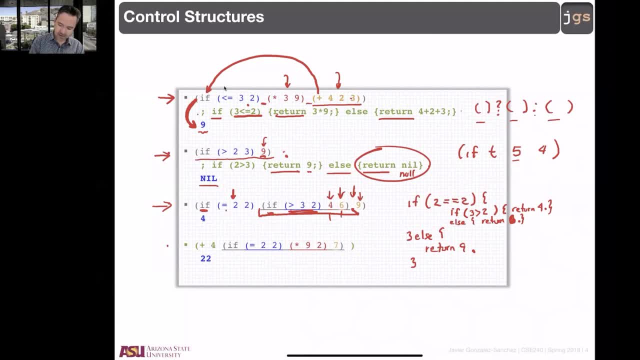 inside of the else. also, if you modify this part, now, the result here is four and the result there is four because, well, think about it, two equals two. yes, we run this if, we run the if and we check the condition: three greater than two: yes, we run this instruction, we run that instruction, we return the value and we return. 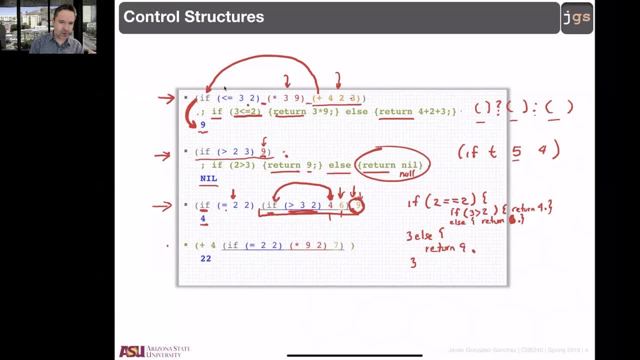 the value here, dot this if and that if is going to return the value to this, if remember one inside of the other, and this one is going to return the value to the interpreter, and that is the reason, because you have that four printed there. every single function returns something, everything. 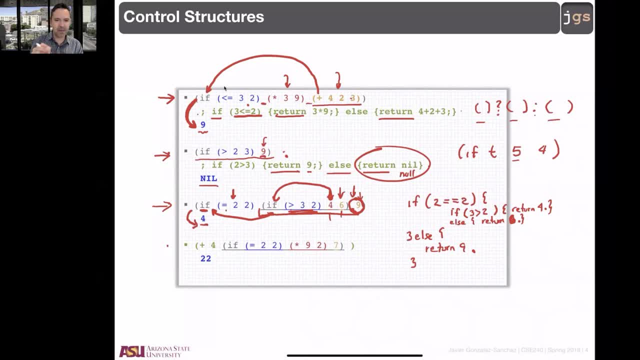 including the if, which help me with the next example. i can have here the addition of four plus. did you notice my addition? have two things: four plus something. only two parameters for the plus. the second parameter is a function. so, as you know, whatever is the result of the second parameter, 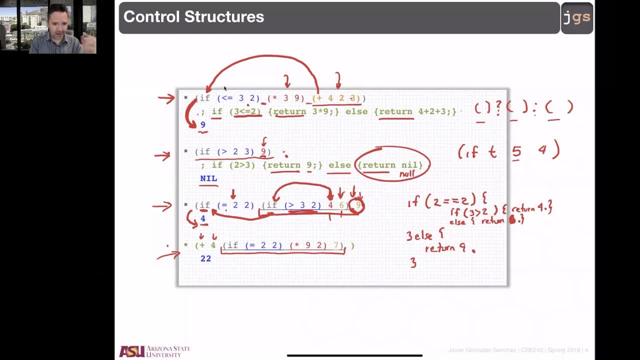 function is going to be added with the four and that is going to be the result of the plus. The problem is what is going to be the result of the second function? Now, my second function is an. if Are you telling me that we can do addition of the number four. 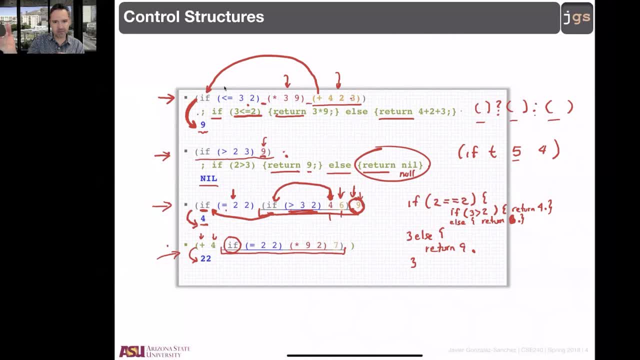 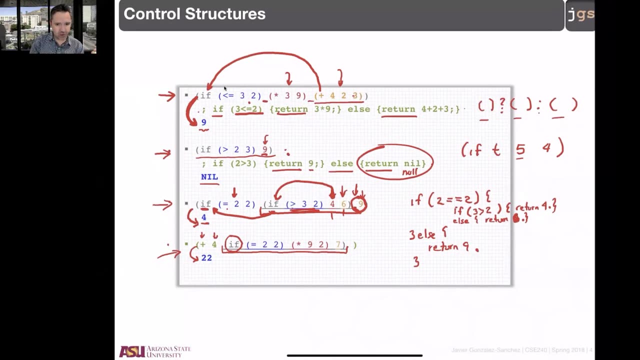 plus an if condition. Yeah, kind of the question mark operator Now here, similar to the previous one, is like: well, I am going to do this function first and the condition is true. Because the condition is true, I am going to execute this one, the red part, not the orange. 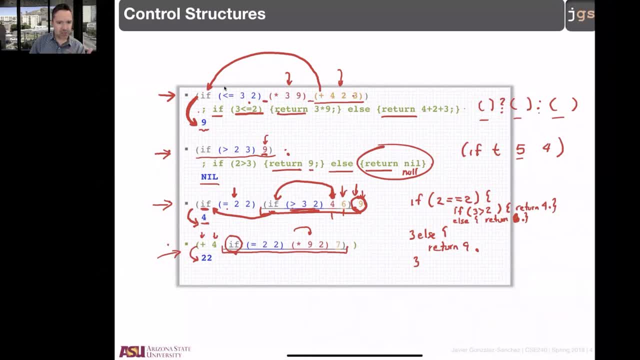 And running the red part is a multiplication. I am going to do nine times two. That is the result that the multiplication is going to return here to the if. It is the one that the if is going to return 18.. And then the plus is going to add the four. 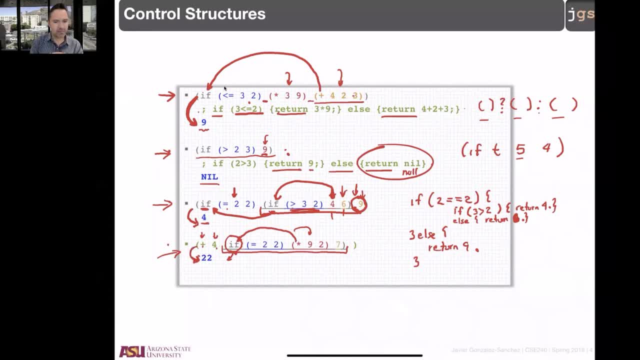 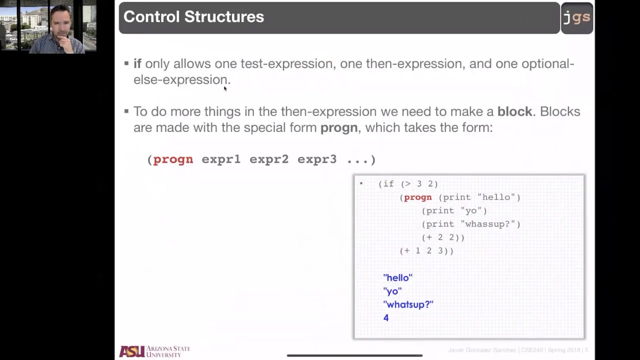 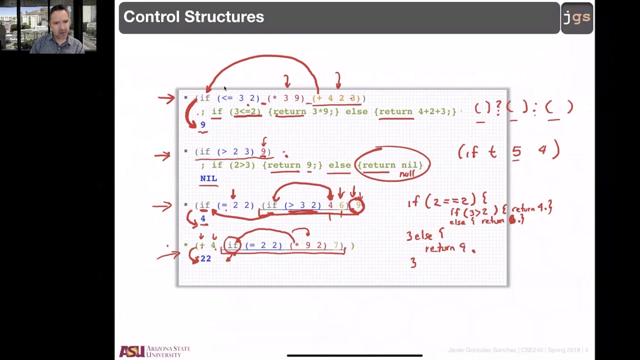 22. And the plus is going to return that as a result, Four plus the result of the if, four plus 18. Done, 22.. The if also return something. Any question? Now, in all these examples, what I did is to do the example of the if. 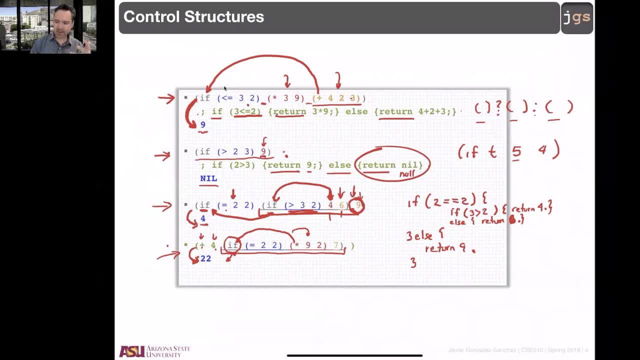 with only one instruction inside. This is basically my equivalent to the question mark operator. the question mark operator- The question mark operator is the same thing. it is an example of the if The question mark operator. one of the limitation of the question mark operator is that you only can have one instruction in the if, one instruction in the else. 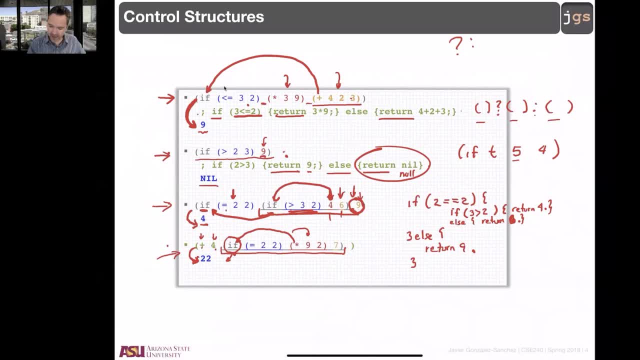 You cannot have a group of instructions, You cannot have what you achieve with the curly brackets. These examples are like that And I am sure that you are thinking like: well, this is OK, One instruction for the true, one instruction for the false. 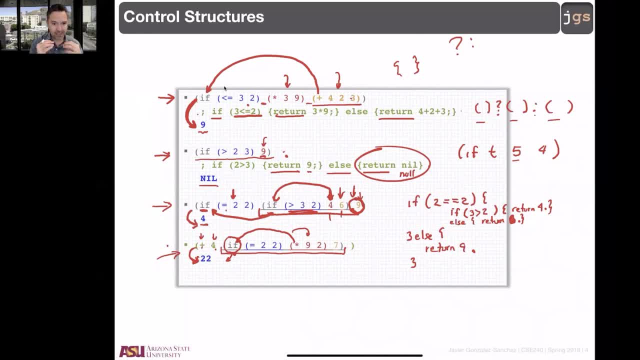 What happens if we want to have several instructions, more than one, inside of the if part or inside of the else part? We need curly brackets, We need to create bodies. Remember, in any other language, the body for the method: curly brackets. 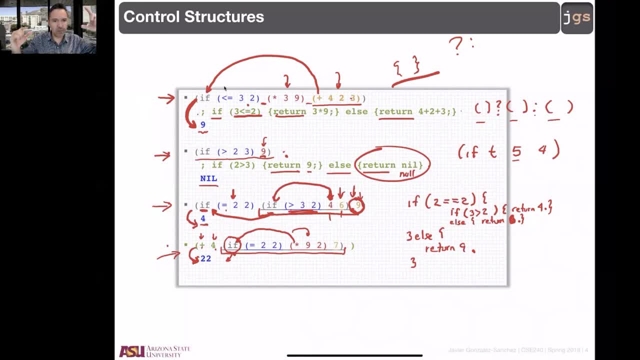 The body for the for loop- more than one instruction in the for loop. curly brackets. The body for the if or for the else: more than one instruction. curly brackets: The curly brackets help us to put together instructions to create bodies In Lisp. we do not have the curly brackets. No curly brackets. 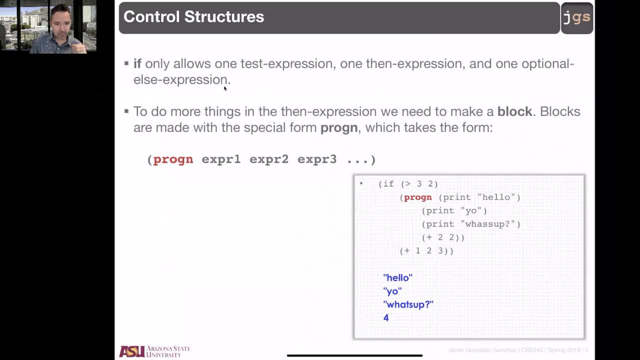 We need something to replace the curly brackets. That something is going to be another function, This function, That one. if you ask me about the equivalence, This is the equivalence. You have a function to replace the curly bracket. Yeah, I have a function to replace this possibility of put several sentences together. 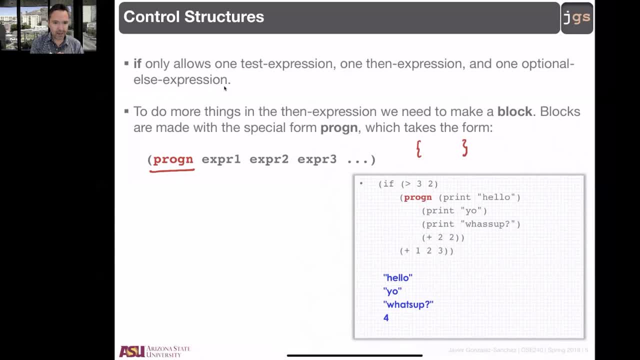 The name of the function, the parameters, The instructions that you want to put together. All the instructions there- And remember parentheses- Is a list with list inside. For instance, this example: here I want to create an if And that if have a condition. 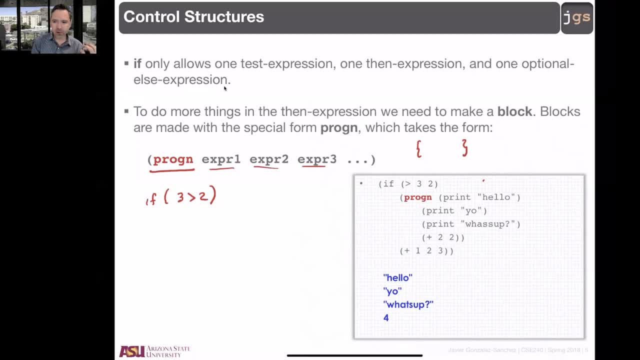 But then in the body. In the body I want to do something like curly bracket, Print something, Print something else And return something. Three instructions: I cannot put both three instructions without these guys, Because if I do that, only the first instruction is inside of the if. 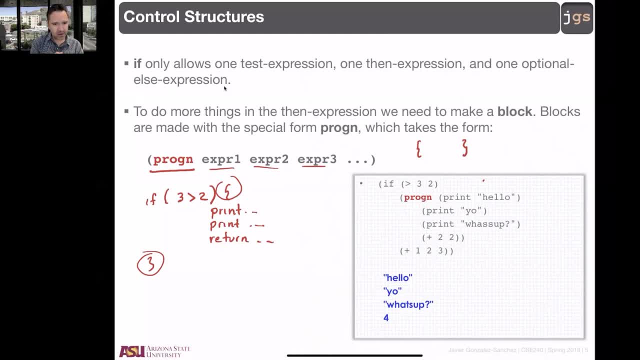 And the other two are outside Right. I need the curly brackets In Lisp, open parentheses And this parentheses is going to close here. Notice that you can use the enters. I mentioned this before. The interpreter is going to allow you to press enter as many times as you need. 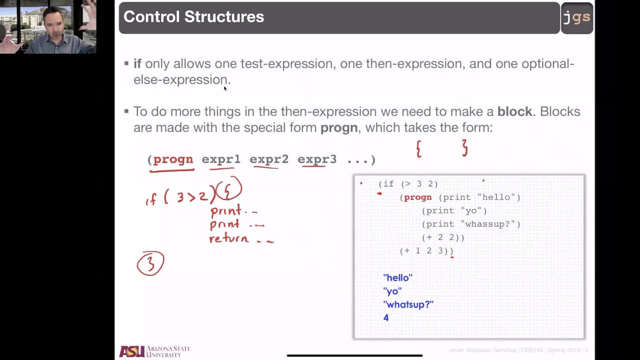 And it's going to wait until all the parentheses are closed before running the instruction. So in this case, this instruction is going to run here, Because that parentheses is the one that closed, the first one that I opened. The instruction is if And the condition as mentioned before, three greater than two. 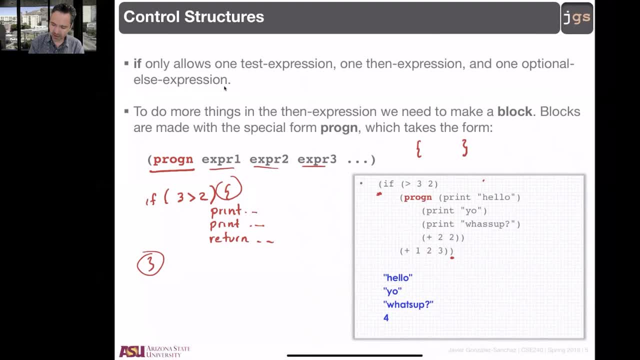 Then the next parameter, the one that usually is here after the white space. I am using an enter. It is not mandatory. I use the enter to use better my space in the slide. But you can create a big line, No problem. 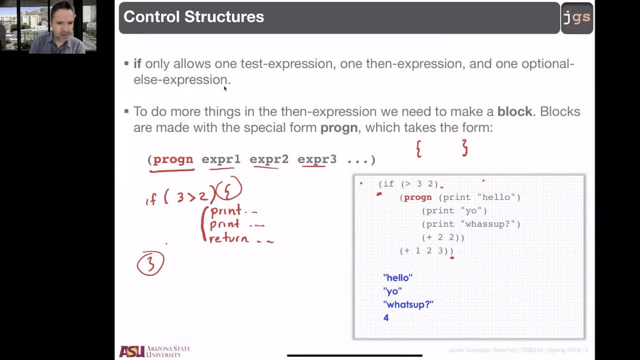 I want three instructions. inside of curly brackets, My curly brackets, Open parentheses. Prog n: That is my curly bracket And obviously that one, the open parentheses, is going to close in some point here. You can imagine that I am opening curly brackets there and closing curly brackets there. 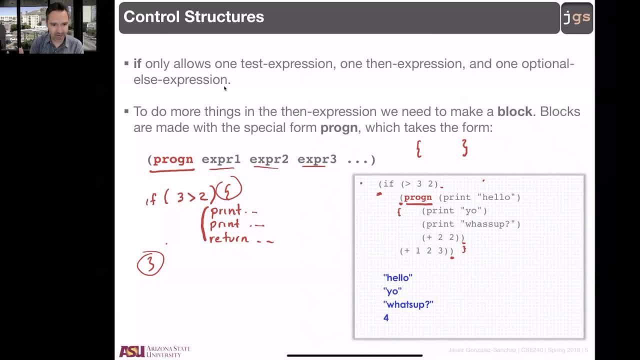 Not because the parentheses, Because the instruction prog n, And inside of prog n I have one instruction, Two instructions, Another print here And the addition In my example. maybe another print here. Three prints and one addition. When the condition is true, it is going to execute this. 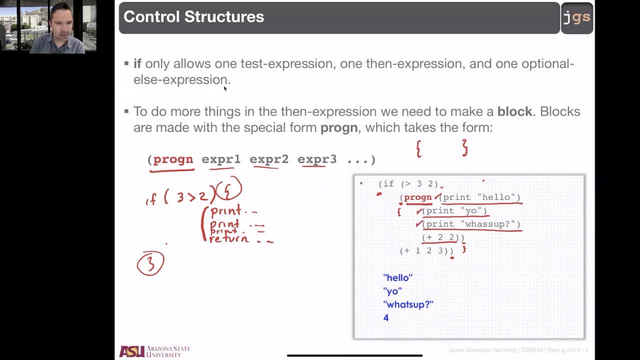 It is going to execute this, It is going to execute this And it is going to do the addition. That is it If the condition is false. If the condition is false, as usual, this parentheses is not going to be executed. 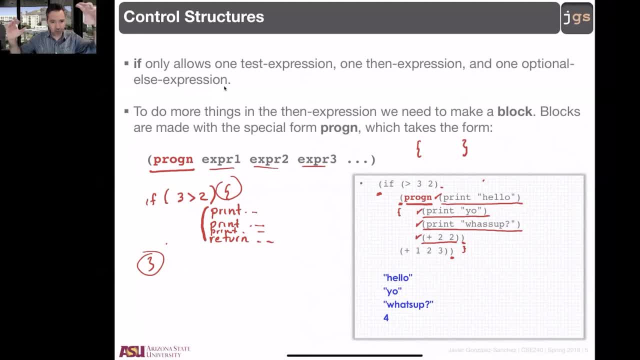 That full parentheses, is the instruction for the true, But it is going to do this one. The last parameter before closing the: if That is the equivalent to have here an else And use Something like that. As you notice, it is not mandatory to put the curly bracket, because it is only one line. 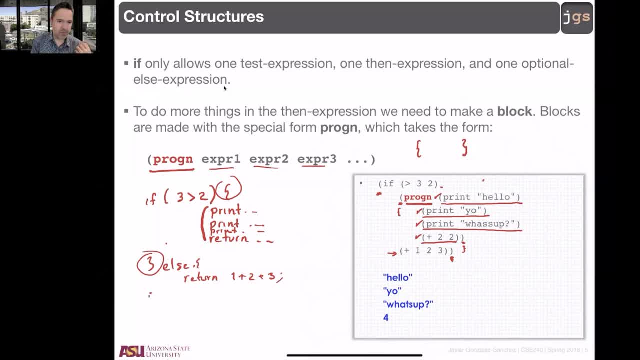 Usually. just to make this clear, you can put this here In the same way: you can use a prog n instruction and put inside only one parameter. That could be the equivalent to use the curly bracket having only one instruction inside. So prog n. 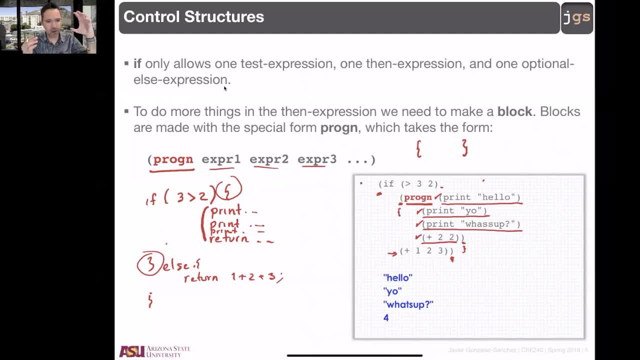 Your replacement for bodies, Your replacement for the curly bracket. This is going to work with the if And we are going to use this also with other things, such as creating methods for the body of the method and loops. Good, Any questions? The return 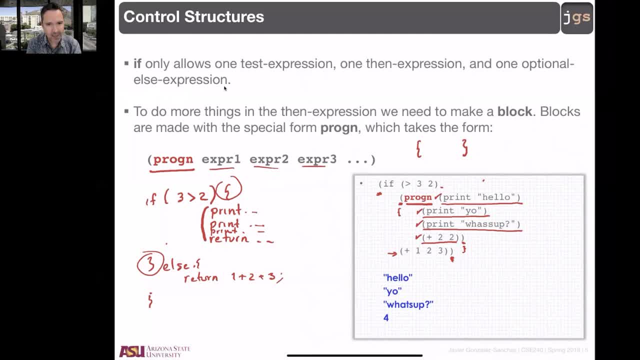 Very good question. What is going to be the return here? Well, In this case it is going to return Either this line or the prog n. The question is, what is going to return prog n? Because prog n has inside a lot of instructions, right? 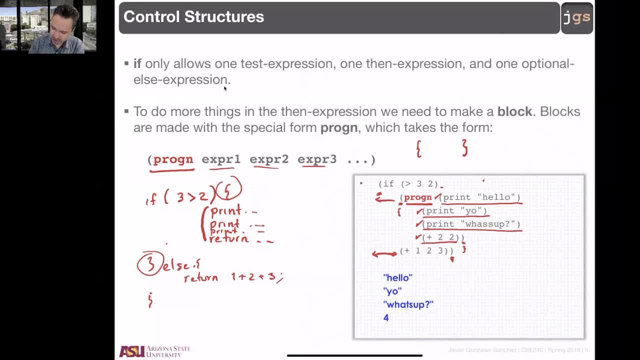 And all those instructions, this one, this one, this one and this one is returning something. All of them are returning something. What is going to return prog n If I have inside four guides, four instructions, Four instructions: returning things Easy? 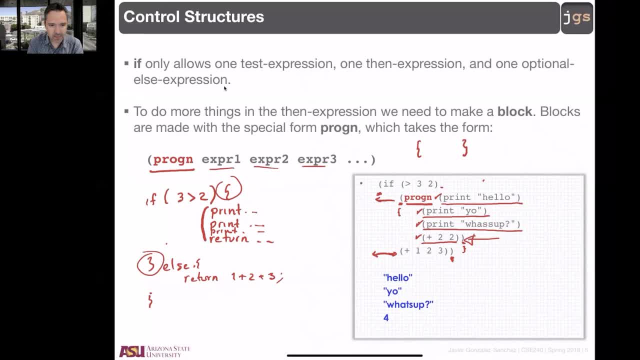 Prog n is going to return the last one. Use the last one. Create a prog n. Create this equivalent to the curly bracket. You can have as many instructions as you want. The last one is the one that prog n is going to return. 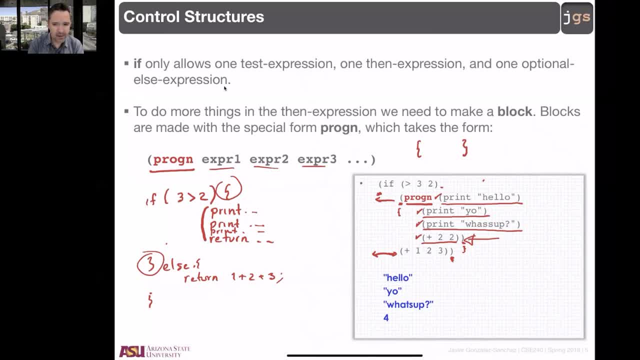 So, in this scenario, All these prints- This is the instruction print here. This is the instruction print here. This is the instruction print here. But then The plus The four, It will not be printed. I do not have a print instruction here. 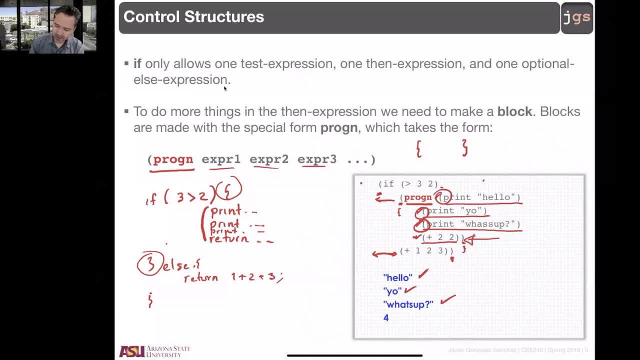 The result of the plus. The last line is returned to prog n. Prog n returned to the if And the if returned. Prog n returned four to the virtual machine. Why four? Because it was the result of prog n. Why four? 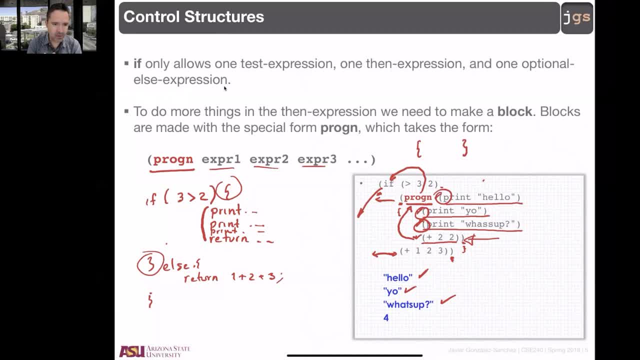 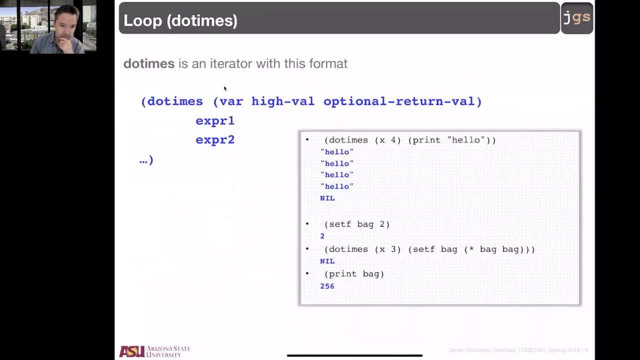 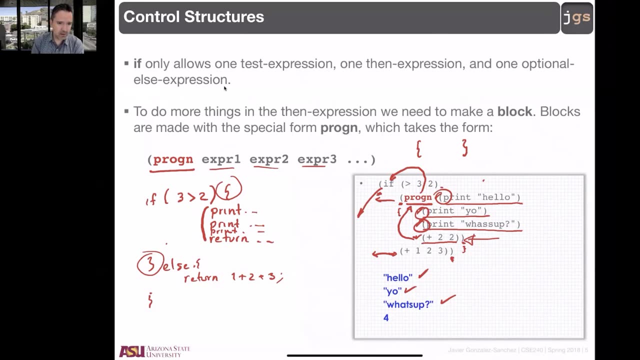 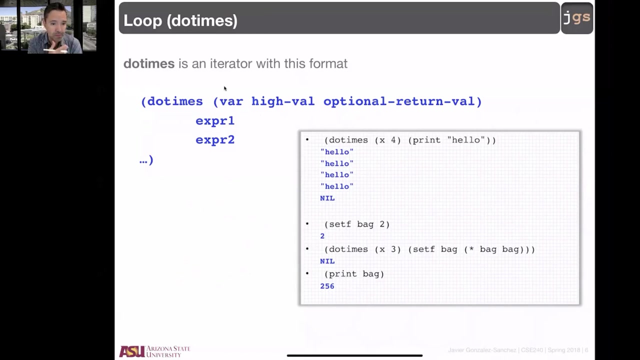 Because it is the last line in the prog n. Good, Okay, So far. Good Oops, Because with this you can create complex if conditions. Now, if we know how to do if conditions, the next step could be how to do loops. 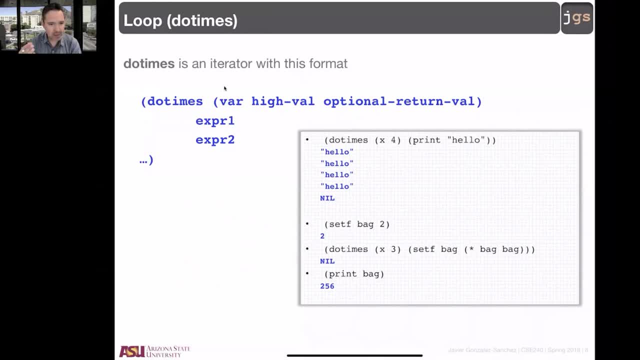 The classical version of a loop in any other language could be the four. It's kind of the traditional one. Four, One number to start, One condition. How many times Repeat For lisp, the main loop, the loop that we usually use? 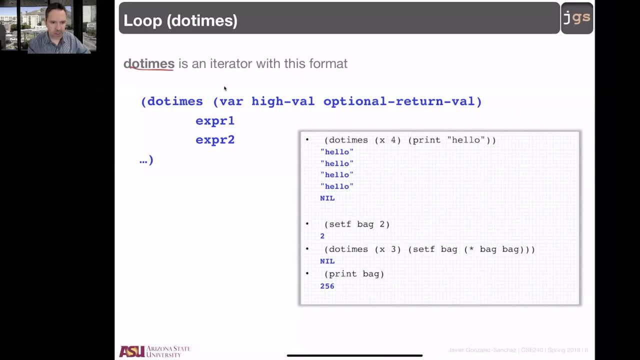 two times, Two times And, as you can expect, it's going to be open parenthesis and the instruction is two times closing parenthesis. So you want to do a loop In order to have a loop open two times closing. 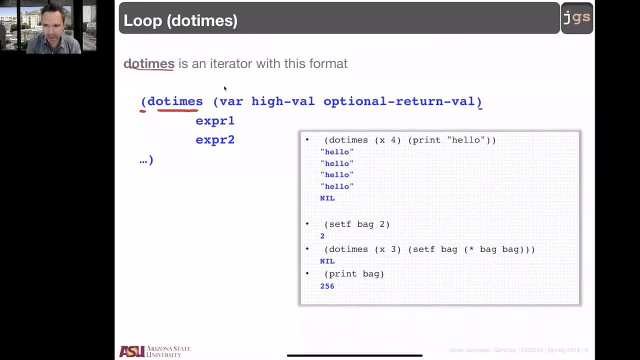 The parameters. What parameters do we need for a loop? Well, for a loop, we're going to need the following: We're going to need one parameter for the configuration of the loop. That one parameter is going to be inside of parenthesis. 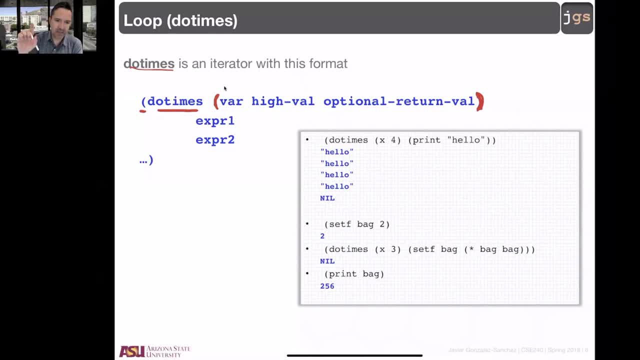 Let me be clear: This is going to be the first time that we're using parenthesis, and the first element is not going to be an instruction Again. the instruction two times have as a first parameter a list of elements in which the first one 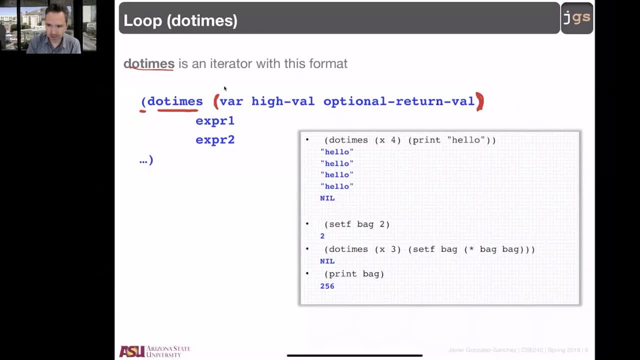 is not an instruction. So this x here is not an instruction, Or the x here is not an instruction. The first set of parenthesis inside of a two times. After the two times, you always, always, always have a parameter, that is: 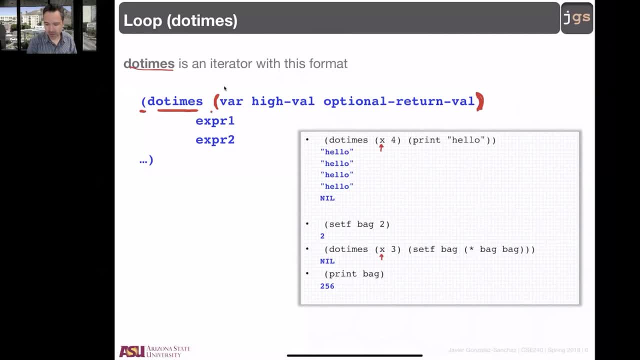 parenthesis open, parenthesis closed: This one, And the interpreter knows that that one is one of the few exceptions in which, even though you have parenthesis, the first element is not an instruction, It's something else, It's a variable. It's a variable. 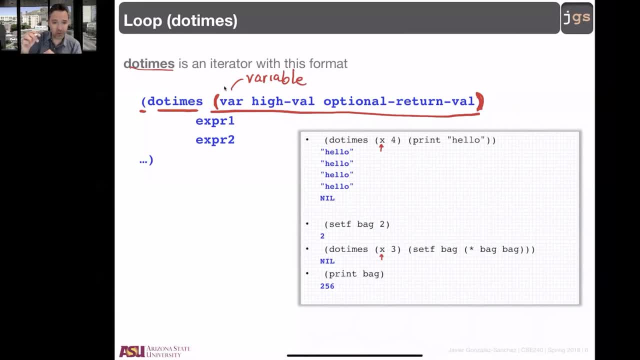 Why? Because for a loop, you need to have a counter of how many times that loop have worked, Just like the variable that you use for the for Parenthesis, two times parenthesis, and the element that you put here is the name of a variable. 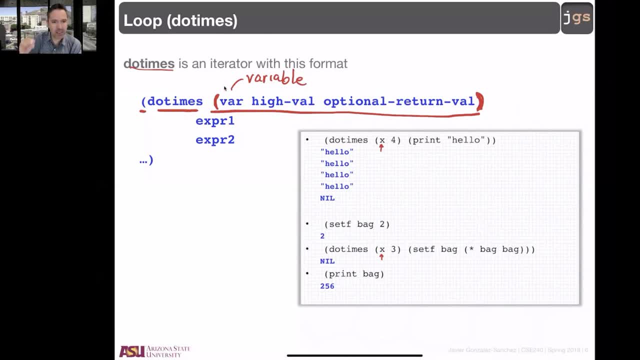 The name of the variable that is counting how many times the loop have run. Your index, your variable i in the for Okay, What else? Well, inside of that parenthesis also, you put the name of the variable. but the next one. 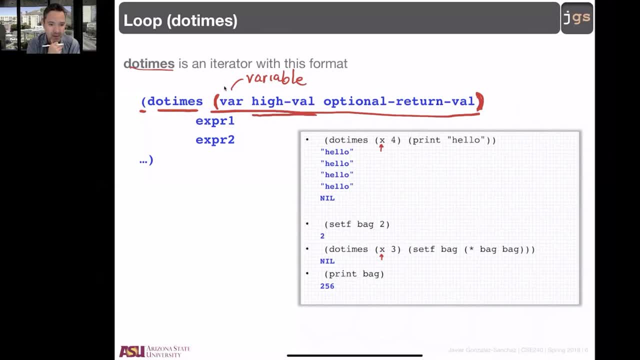 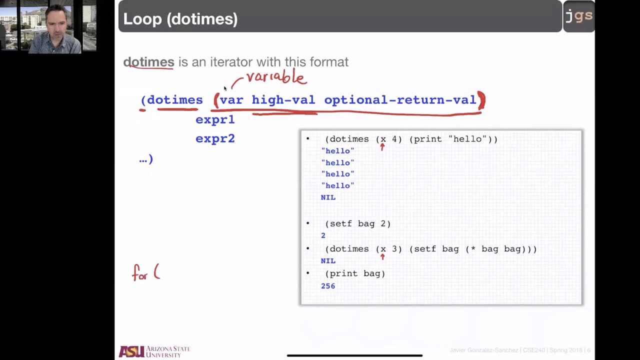 is the higher value for the variable, Like the value that is going to stop the loop. It's kind of a for in which you have a variable like this And then you have the variable lower than some kind of value here. That is the value. 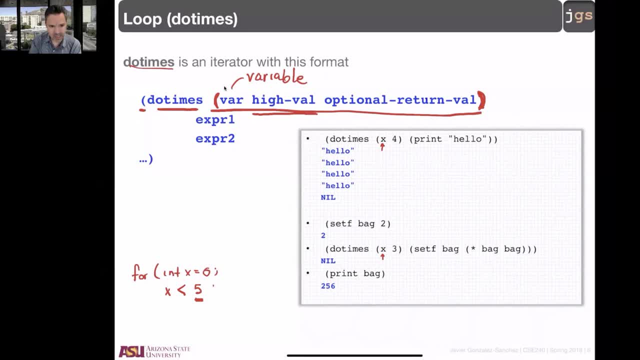 that I am talking about. In Lisp, you will do open parenthesis, two times open parenthesis, and then the variable x, And then I don't care about equal zero, I don't care about the lower than five, That is obvious. 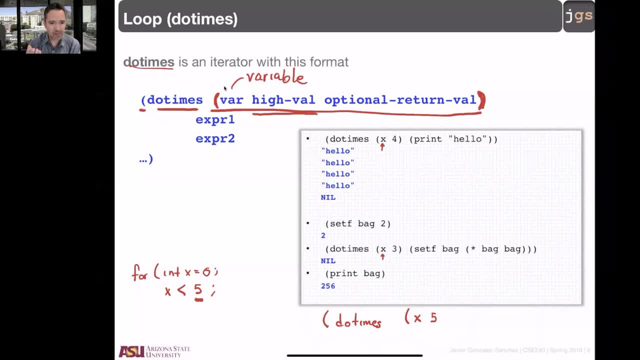 Five. Why five? It's the number. It's the number that you want to use to stop the loop. It's the number of times that you want the loop to roll. That is the information that I need as the source code. Two times. 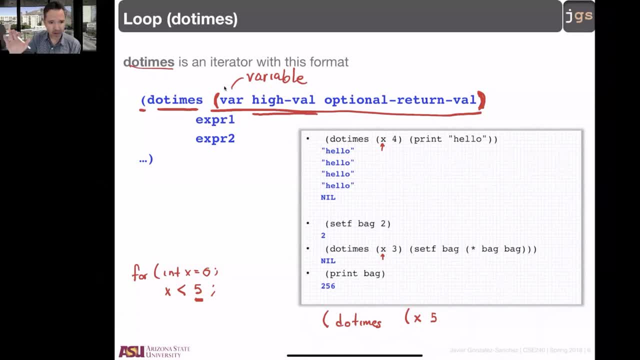 parenthesis x, five, And you can stop there. You can use close this and this is the configuration of the loop, The variable that I am going to use, the name of the variable and the top value, the higher value. 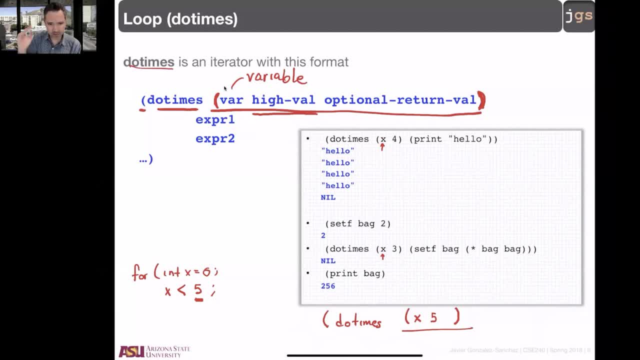 for that variable. When that variable has that value, the loop stops Again. it's the first time that this thing is not an instruction. It's whatever name you want to put to your variables. I am using x, You can use cat. 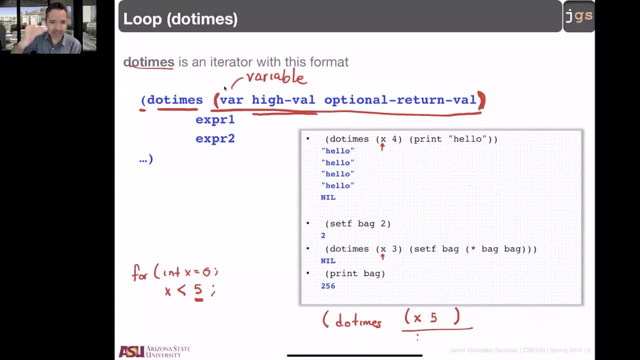 dog, computer phone, whatever It's the name of your variable. Whatever name you want to use is not a function Now optional. you can add one more thing here to make it three elements inside of the parenthesis. Which elements? 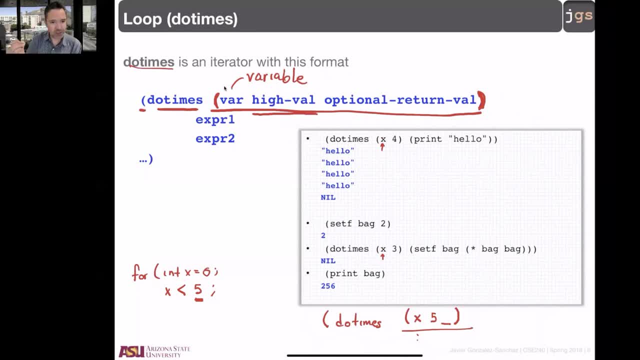 Well, dot time is a function. Dot time is going to return something, Something, What, Whatever you put here, Whatever you put, there is going to be the return value of the function dot time. Did you notice? For some functions they return. 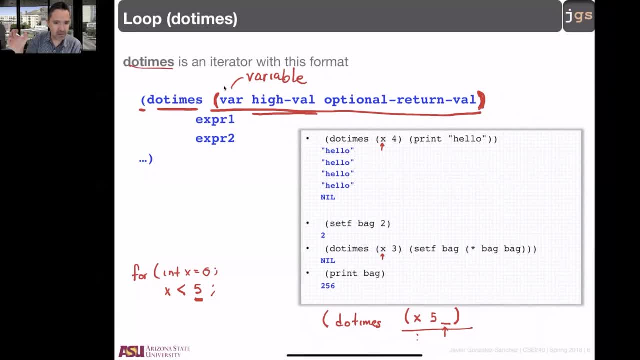 whatever is the return value of the function dot times, Did you notice? Whatever is the result of the operation For others, like proc n, they return. whatever is the last line inside The dot time? The dot time is special. The dot time is going to return. 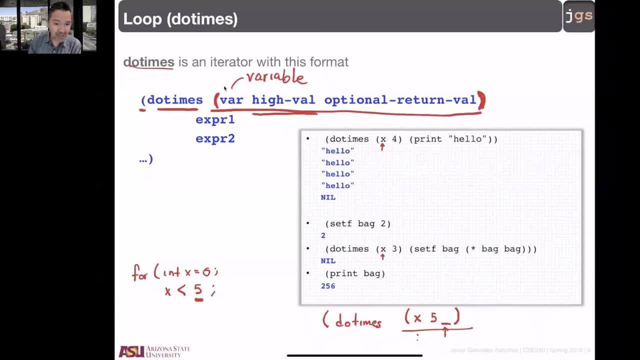 what you put in this place, The last value of this list. So if I put here a five, this for loop is going to return a five. If I put here hello, this for loop is going to return hello, whatever Usually. 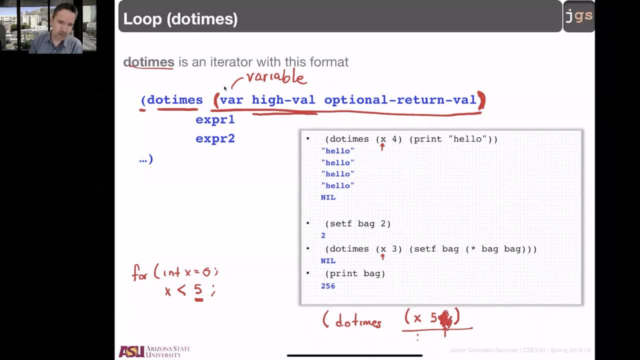 you put nothing. So usually you're going to do like this: Parenthesis, the variable and the top value. I mean I don't care about the return, And if you do that the return is going to be null. 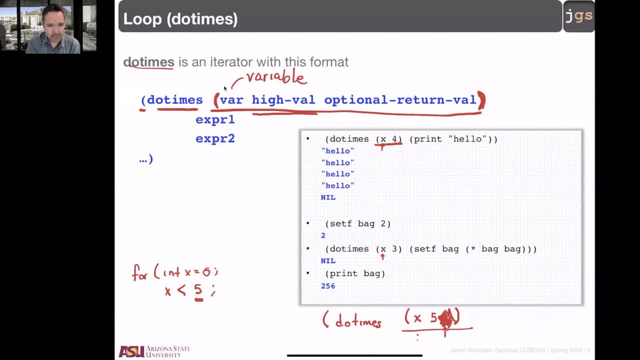 That nil. there is the return value of my loop. So if I put zero it's going to be zero. So the return of my loop, the loop is returning nil. It's not because it's an error. Nothing is bad here. 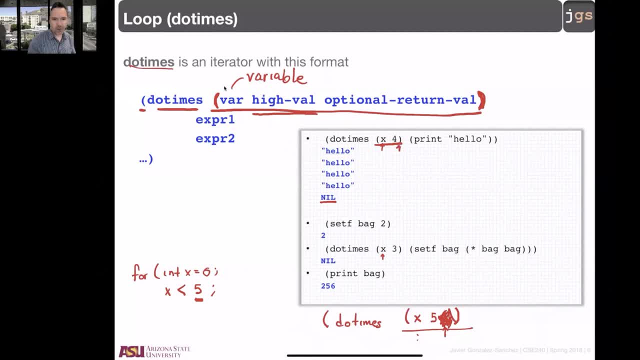 It's because, well, you didn't put the return value, So, when you didn't provide information, that information is nil. You know what happened with the if-else. So, moving forward two times, parenthesis, with the variable and 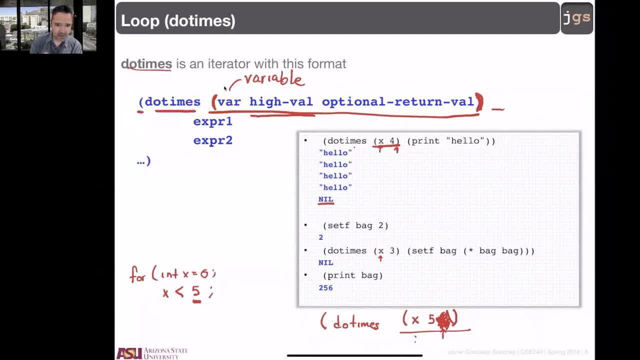 next. after this, all the other are the instructions that you want to execute. All the instructions. It could be only one, It could be a proc n, or it could be used several instructions or multiple times include the equivalent of your proc n. 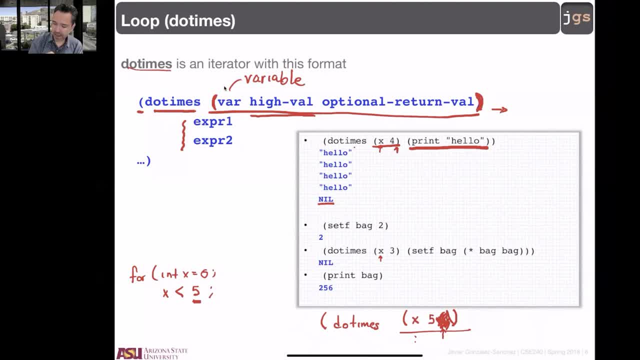 this grouping instructions here. So now, hopefully this example is clear. It's like: two times, the variable is x. I'm going to stop in four. So this loop is going to run four times And the loop will print. 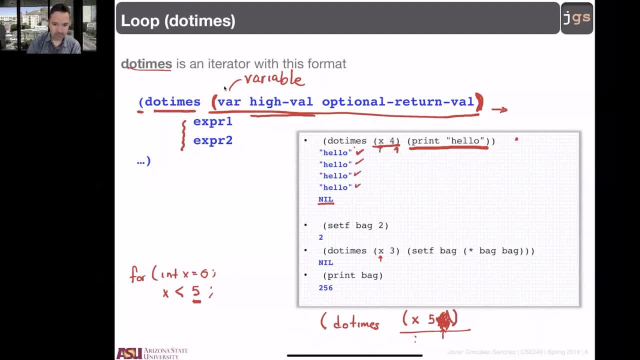 hello, one, two, three, four times, And then the nil, that is the return value of the two times. that then is printed on the screen Done. Now there is an issue here. Sometimes you're going to need variables. 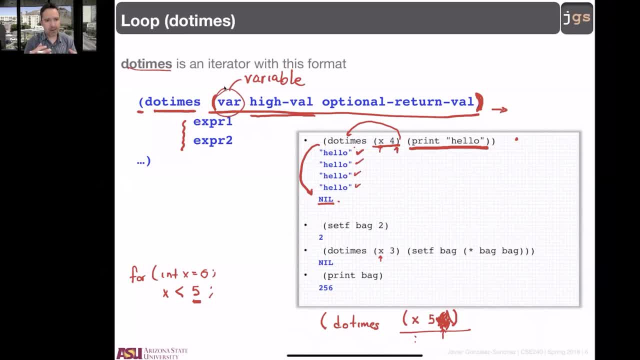 In fact we are starting working here with variables. And if we start working with variables, as you noticed there, I only put the name of the variable. I do not have data types. That is fine. But also I am thinking like: 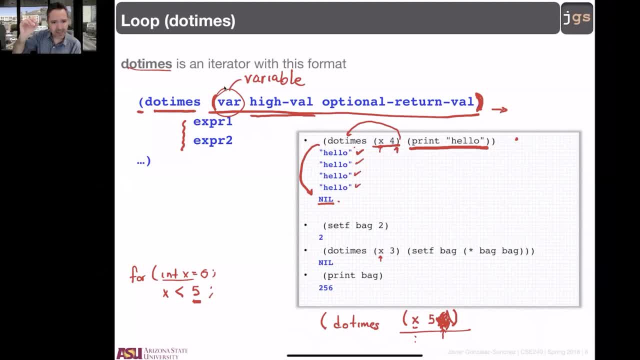 what if I want to provide a value for the variable? What happens if, for any reason, I need a variable and I want to put a value inside of that variable at the value? However, my problem is, if this is the variable and I want to. 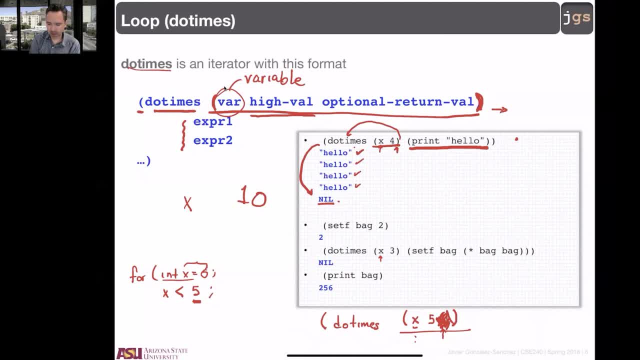 put a value 10,. usually previously, what I used to do is, like in math: variable equals the value. I already know that I cannot do this. Moreover, here these two- the name of the variable and the value, should be: 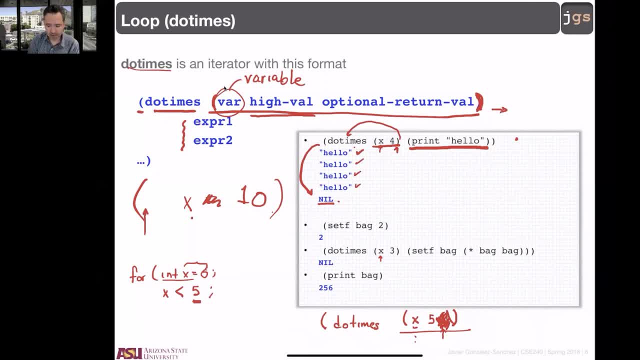 together and the operation goes here. So something that is equivalent to the equal should be there, then the variable, and then the variable should be something else there. I need a replacement for the equal that I used to use for the assignment. The replacement. 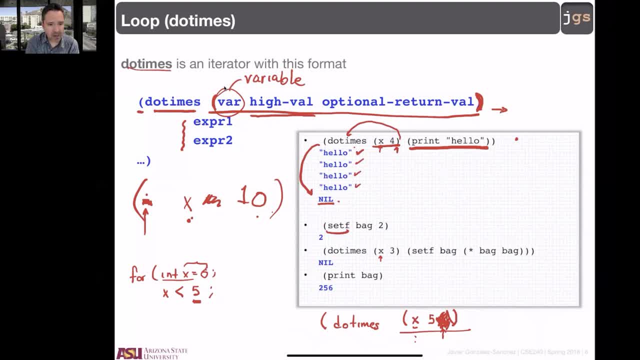 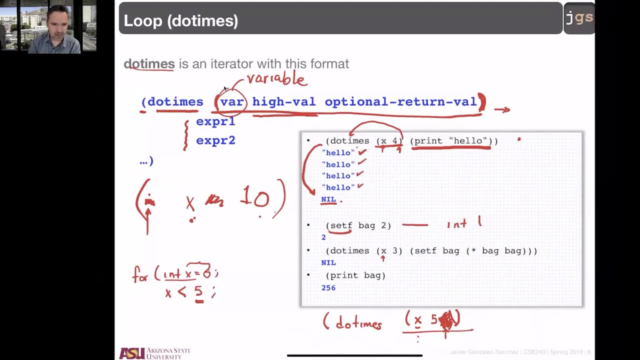 for that is going to be this guy. ZF is your replacement for the equal in an assignment. So the name of the variable is Bach and the initial value is two. This line here is that equivalence. How do you know that it's? 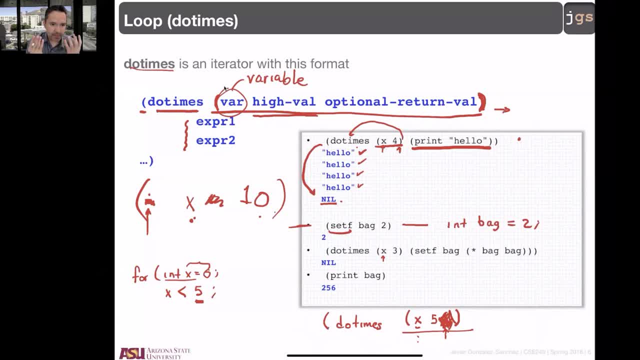 an integer. Well, I am storing as an initial value the number two. so, whatever you want, I do not need to ask you about your long sign it or unsign it. You use integer Equal ZF. Yeah, this one is kind. 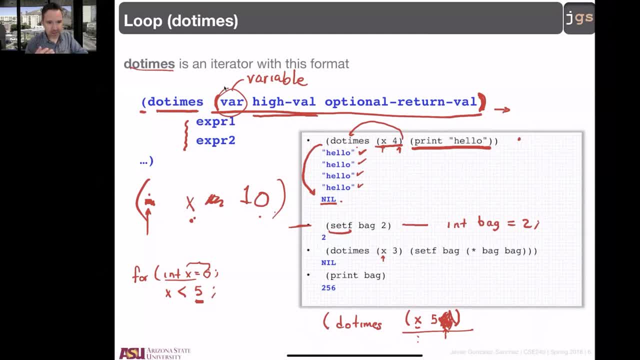 of a little bit weird, but ZF is like the sectors in the next white spaces. Okay, so this program, that line, create a variable. By the way, when you create a variable with ZF, that variable is global. 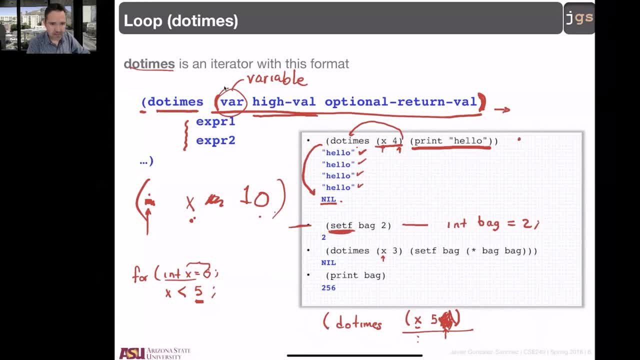 Global. Yeah, you create a variable and you can continue using the variable, and there is going to be another instruction for local variables. assignation of local variables, Don't worry So. ZF global- This one back equal to a. 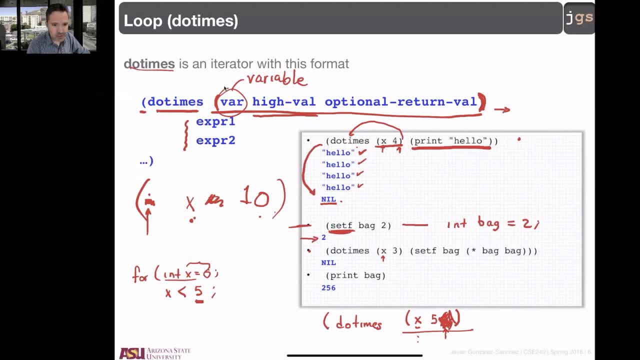 global variable back with the initial value two. Okay, next another example. So this is the same number that ZF is going to return, which makes sense. It's like the print returning the same thing, that is printing, Anyway. 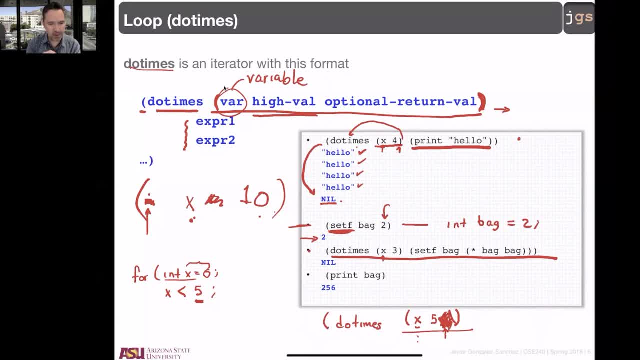 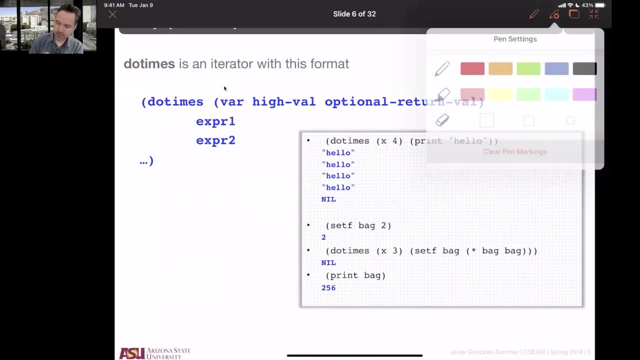 next add two times. Two times, If I ask you to do the same thing here. in that for loop, it is clear that I am doing an integer variable back equal to here, And then I move forward to a variable x as the control. 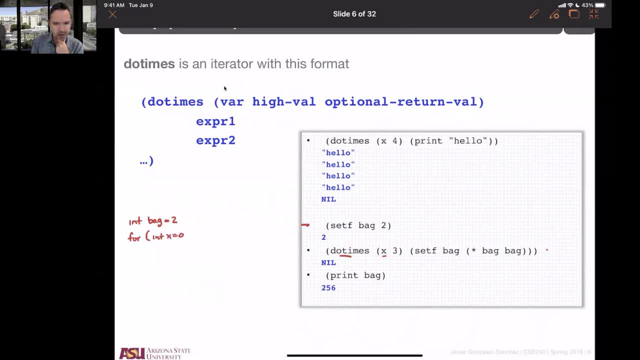 variable, The top value or the maximum value for that one. the number of execution that I want for the loop is only one instruction, Obviously, the variable should be incremented. One instruction, Yeah, And the instruction is correct. Set back this set. 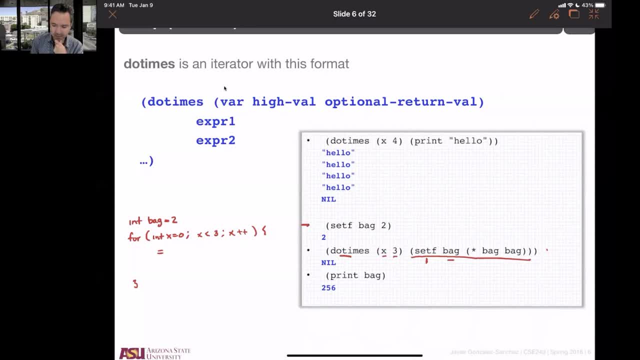 is the equivalent to the equal of one initial and the number of units. So this one is like this one, And these two times is like this for loop, And therefore something is happening. Something is happening, This multiplication is happening and is. 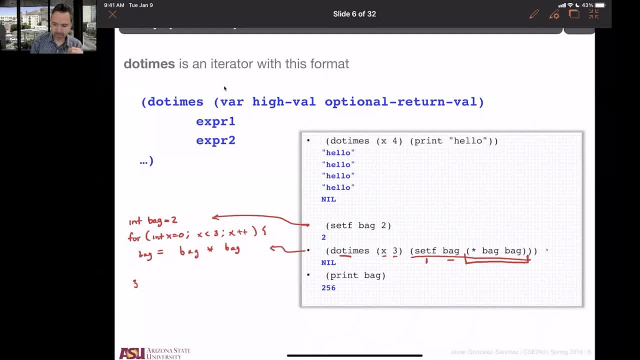 being stored the result in this variable. Why this nil is printed there? any error, any problem with my for loop? no, it's just because the return value should be here. remember x, top value, the return value. i didn't put any return value. this one is going to return. 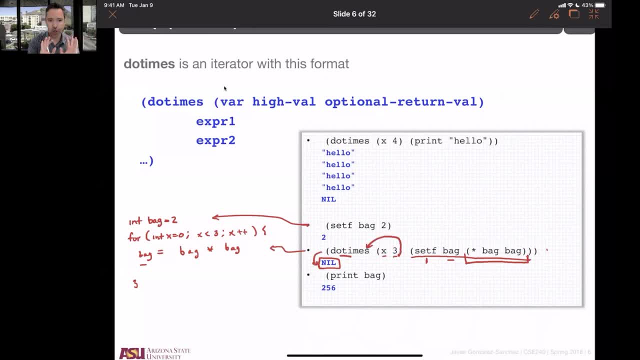 nil, no return value. you want to return something, that something should be there, the third element in those parentheses. if not, it's nil, no problem. this is a particular case in which my result is not something that i want to return, but something that i am storing in a variable. i want to print my variable. i want to print. 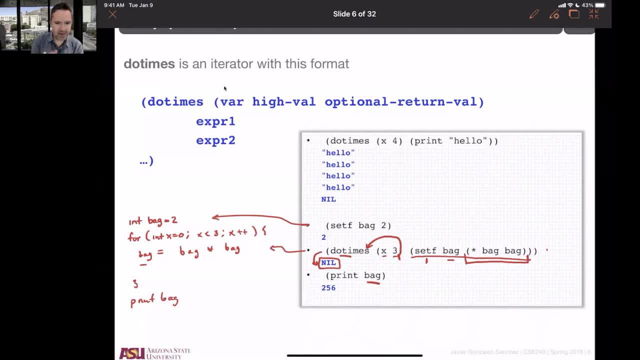 you back and i am using print. but if you go to java system, open ln, if you go to c plus plus c, out, etc. so print back. it's a global variable. if i print the variable, it's not going to be the two, because i use the variable inside of the four. 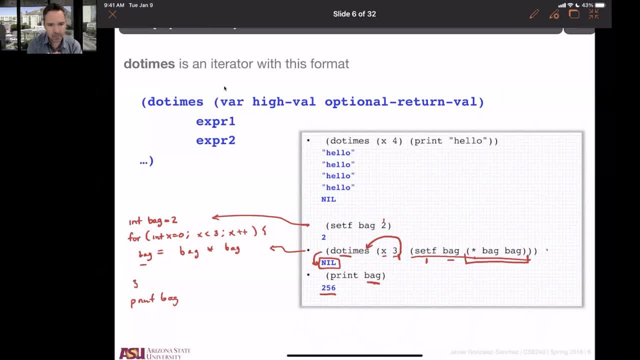 two, five, six. we start two times two and we store, and then four times four and we store, so on for loops and global variables, for loops and assignations. hopefully clear any questions? so far good. so now we have conditions and now we have loops and we can start doing. 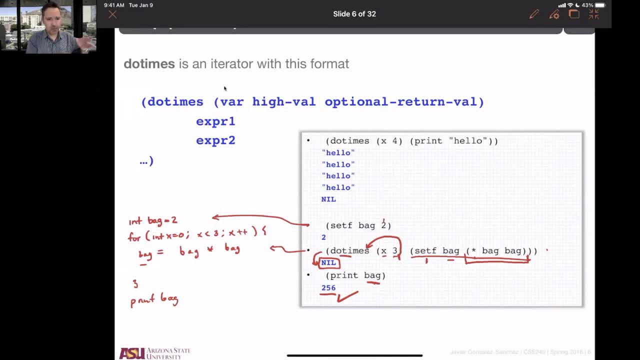 programs a little bit more interesting, like those programs that you did in csi 110. right, the best programs that you did there with java was programs with conditions and loops. yeah, we're going to have breaks and continues. we're going to talk about it now here with this. 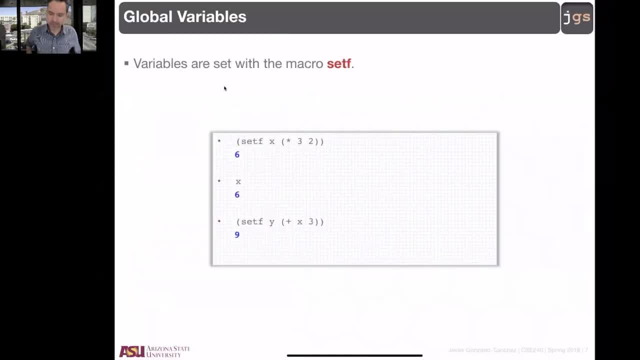 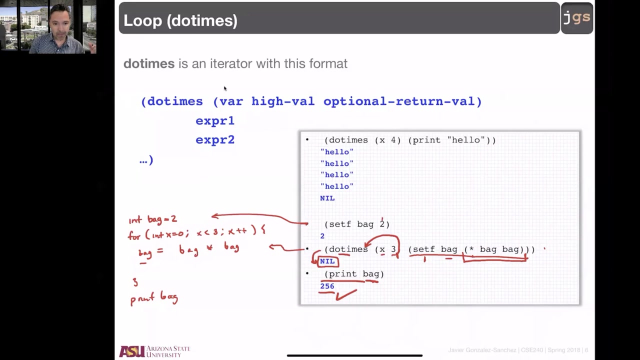 what can we do with this program? big parenthesis, the set, the variable, the value. if you put in one program the name of a variable alone, automatically the system is going to print the value. so just as a notice here in my previous example, i will do print back. 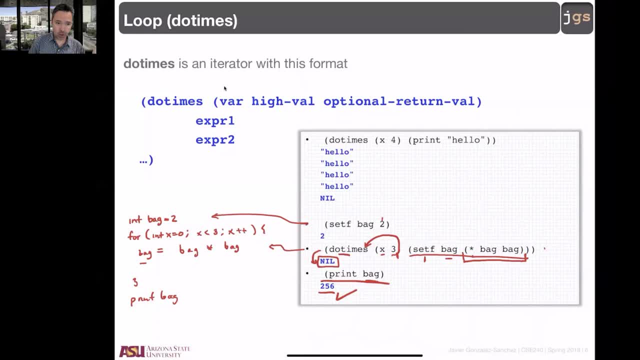 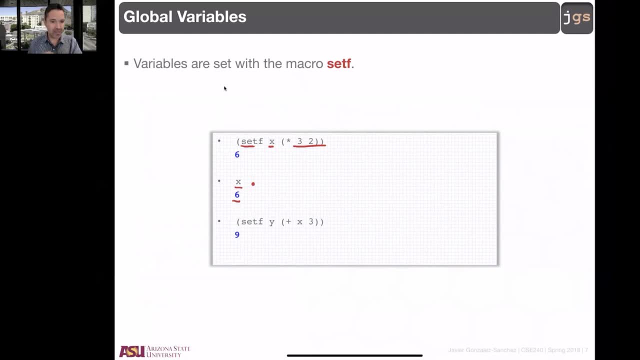 press enter and i can have the result. or you can do only the name of the variable enter and automatically, if you provide the name of variable to the virtual machine, what the virtual machine is going to do is to print the value of that variable. so you can save time with the parenthesis. 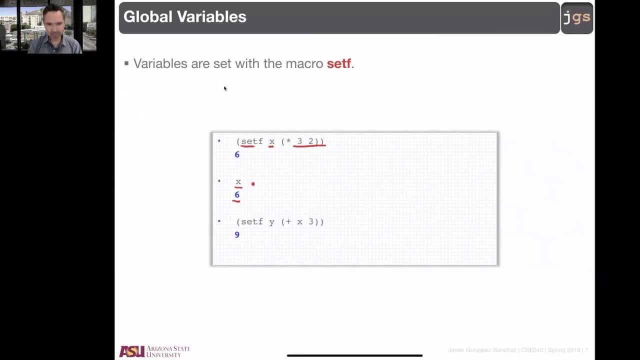 on the print. eliminate that and use the name of the variable. and that is the equivalent to using the value. and in the common prompt is to print the value. Similar if you are returning something, For instance, you can have an if you can have. 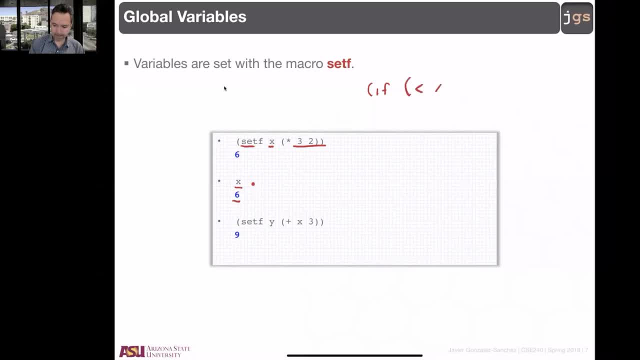 a condition. you can use variables and you can do something like this: If you have only the name of the variable in the console or in any of the instructions, what is going to happen is in that example here, if the value of the variable x is lower than the. 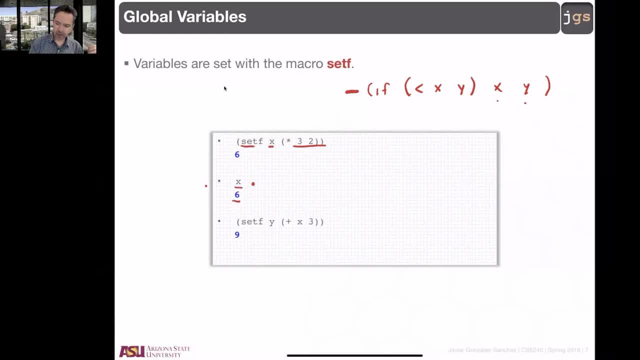 value of the variable y, return x And x. the value of x is going to be what this print return and therefore what is printed. So this is the programming lisp: to return the smallest variable or the variable with the smallest value, If x lower than xy, x space y, Something that you need to remember. 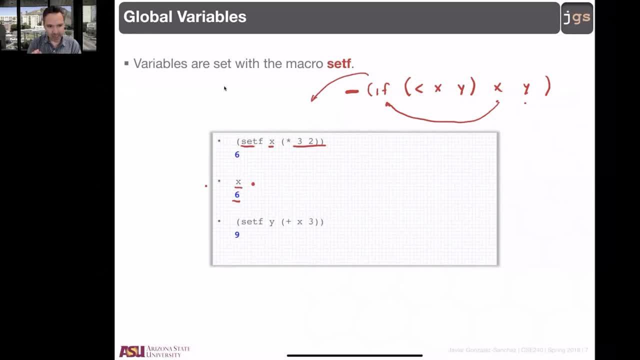 we do not have a return instruction here. The return happens automatically. There is not going to be a parenthesis return or something like that. If you put here a variable, as in the previous examples, we put numbers Automatically. what we are. 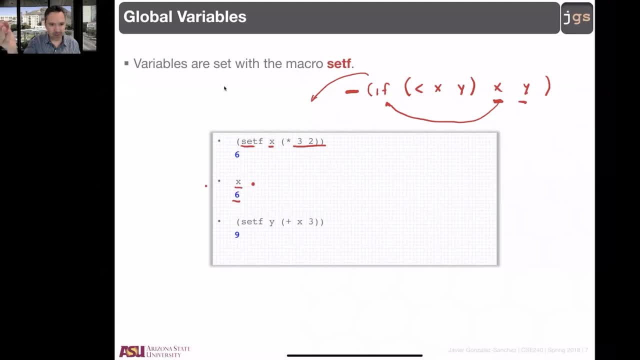 asking is for that variable, the value of that variable or that value directly to be returned. So examples like this are coming. Anyway, obviously, if we want to do something like this, that one is y equal x Plus three And hopefully that is clear. Set f is the equal First. the name of the 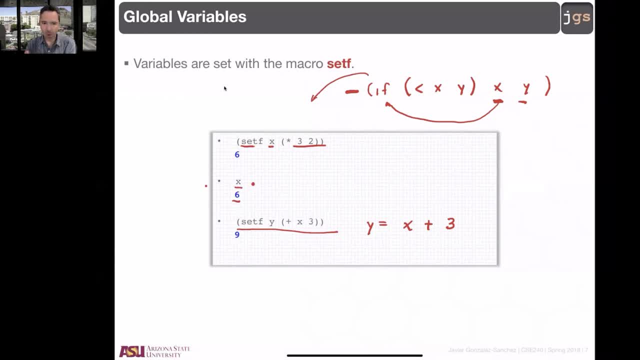 variable And then you can have whatever you want In the previous examples: a value directly, like in the examples that I showed you with the loop, But you can put there instead of the value another function And all the operators are functions. So you can do addition, multiplication. 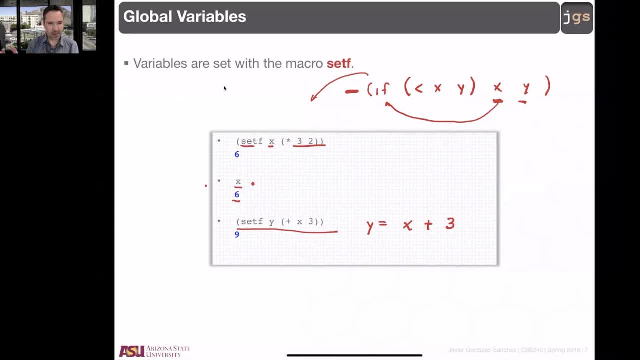 division, whatever To store that, But also parenthesis. Set f a variable. That one is going to be the value, So it's going to be the value. Can I use an if as the possible value for the variable? 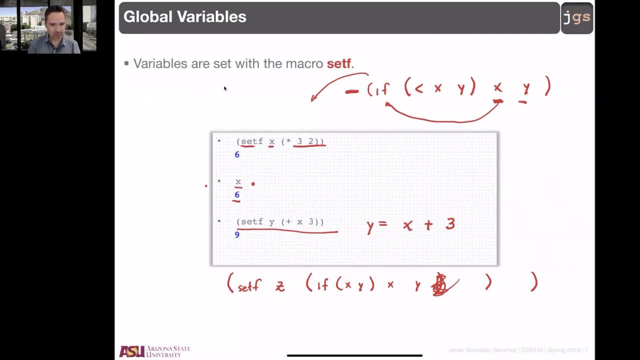 Yeah, the if returns something, So that something is going to be the value for the variable. Moreover, connecting with the previous example, if the if is this, if that is checking which is the lower or greater value between two variables, What I am doing is just like the small value in these two variables is going to be stored. 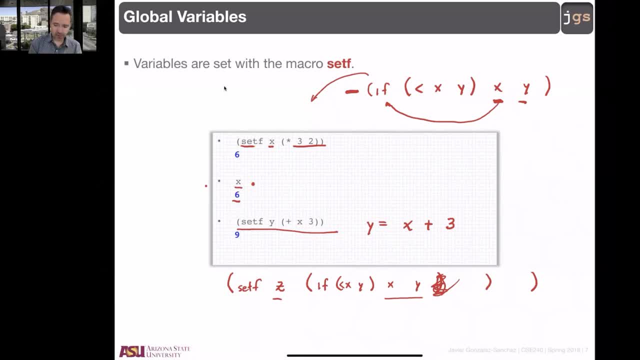 in C. Obviously, in order to make this program to run, I need to create those variables. So somehow here I need to use a set F, another one and I need to create the variable X. Okay, Let's maybe put some initial value, if you want, and in another line. 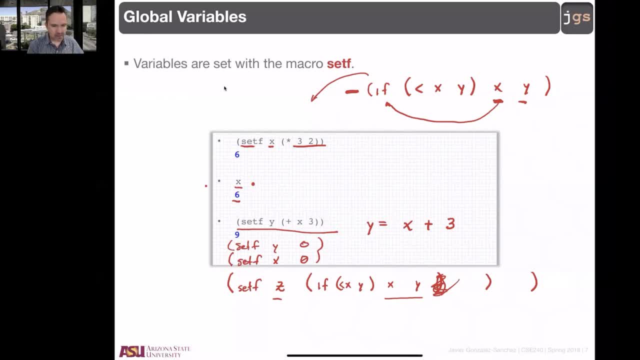 So this is looking more like a program. Now my program is three lines: two lines in order to create variables, global X and Y, and another line to a store in another variable, another value that basically is the smallest value from the previous two. In this example, both are zero. 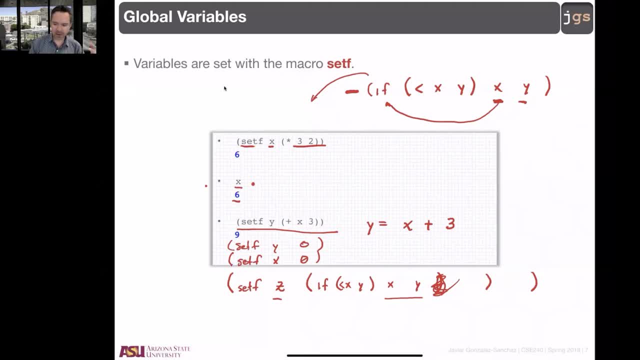 So my third variable is going to have also zero, but you can imagine what's happening here. I do something else, call functions do the process of some data or something. We're going to play with that. But this is one program. 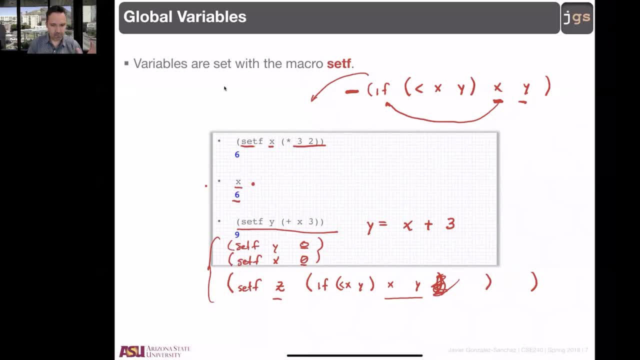 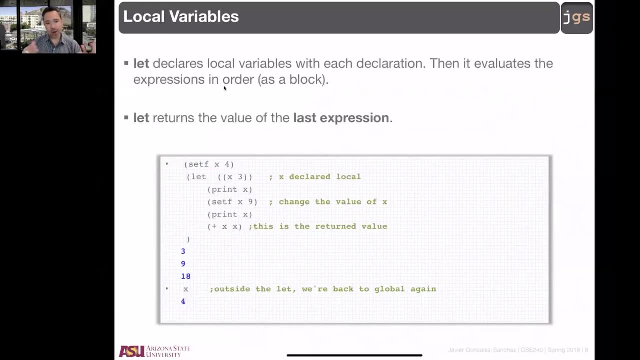 And now we have variables, global, and this guy, in the same way that the loop can be used to return something can be used in an assignation. Good, Okay, Let's see what we have here. Local variables, It's like: well, we have is, we have force, we have global. 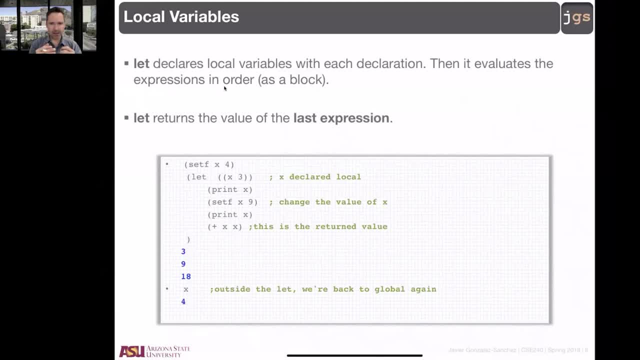 What about the locals? The locals? Let's review this. The local variables are those variables that are created inside of curly brackets and only exist inside of those curly brackets. Think about it: A local variable Is inside of the curly brackets of a method and only exists when the program is running. 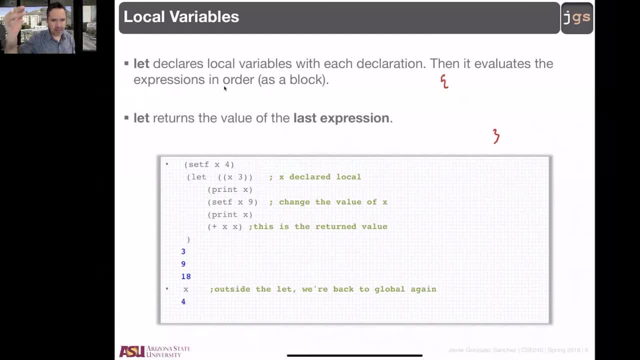 between those boundaries. Parameters are a special case. Parameters are considered local variables. Parameters exist in the body of the method, right, But also, if you think about an if in Java, in Java, even though the if is inside of a method, 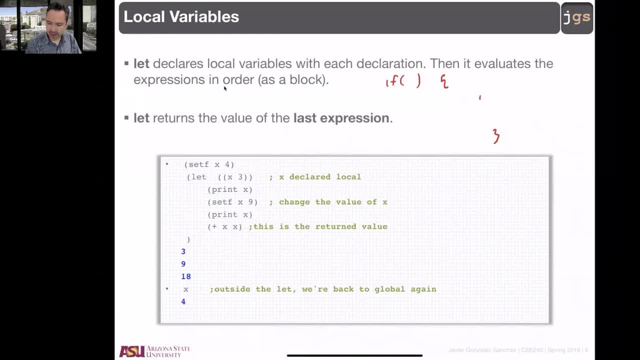 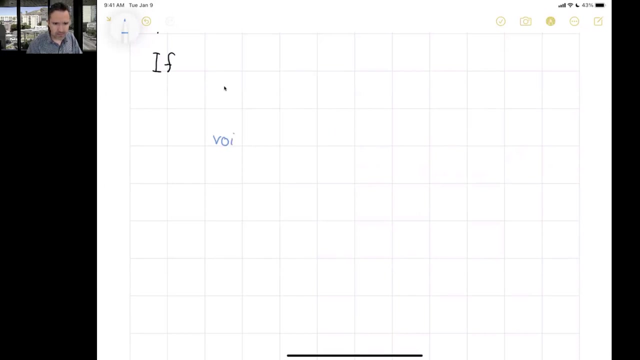 If you have an if And you create a variable here, can you agree with me that this variable is going to exist only inside of the if? Have you tried to have in Java a program in which you have a method inside of the method? 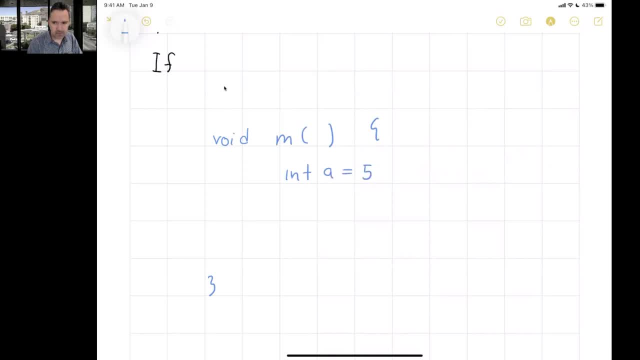 you have a variable, Inside of that, you have a condition. Doesn't matter the condition, And Is this possible? Can we have, Moreover, a global one? the global one and the local one? yes, of course. what about another local one, not in java, c, c, plus, plus. 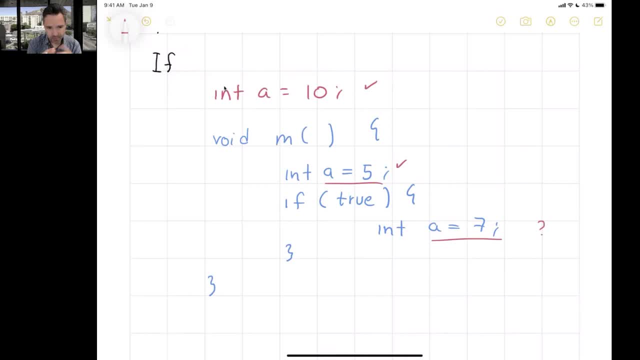 the scope- some languages is like scope. this can be possible because this one exists between these boundaries. if you are inside of the, if this guy is the one local, if you are not inside of this but you are inside of the method, this is the guy that is local, And if you are not, 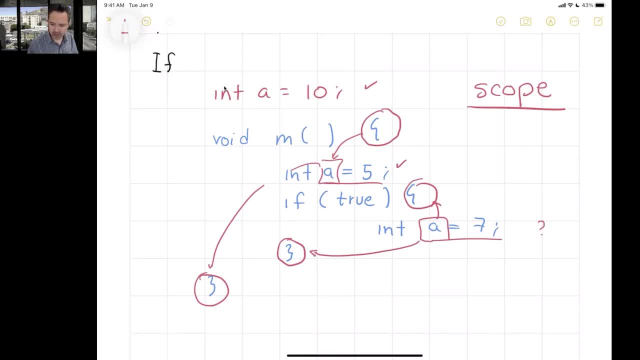 in this method. if you are in another part of the program, this guy is the one that you can use. The scope of the variable. The variable lives inside of a particular zone of your program. This is the way Lisp work. This is the concept that Lisp have for local variables. 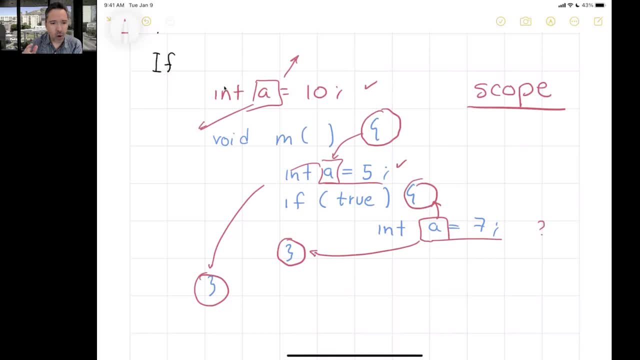 Local variables are not exactly only the variables inside of a method. A variable can be local if that variable is inside of the body of whatever, Inside of the body of a loop. a local variable to the loop Inside of the body of an if is a local variable to the if. 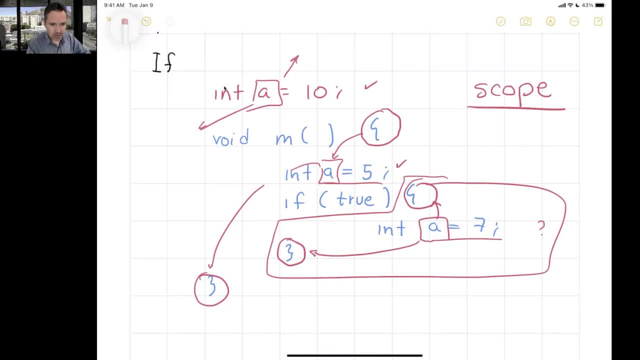 Inside of the body of the else is a local variable in the body of the else. That is going to be the concept here. So local variables, they are more than use the variables inside of a method. They are the variables inside of curly brackets inside of a body. 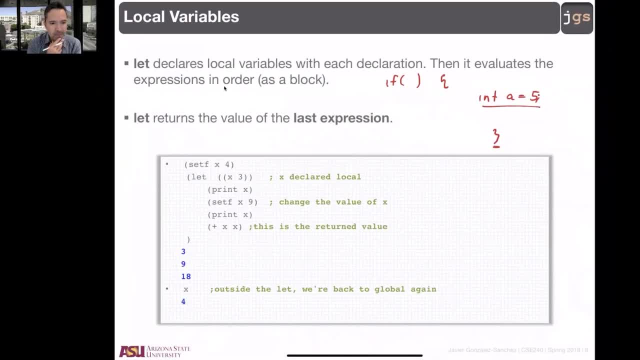 When you want to create a body, you use proc n. We already talked about it. If you want to create a body and inside of that body you want to create local variables for that body, your instruction is: let Let is a similar idea that proc let is a similar idea. that proc let is a similar idea that. 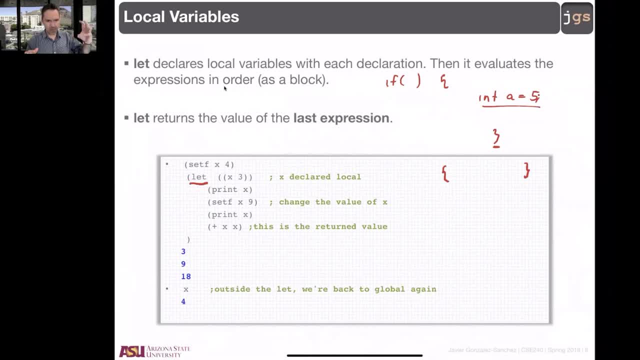 proc let. isa is going to be like your curly brackets. It's going to allow you to put the instructions together, But you can create variables here and those variables can be used for any of the instructions, but only inside of this bracket, Only for any of the instructions inside of this let function. 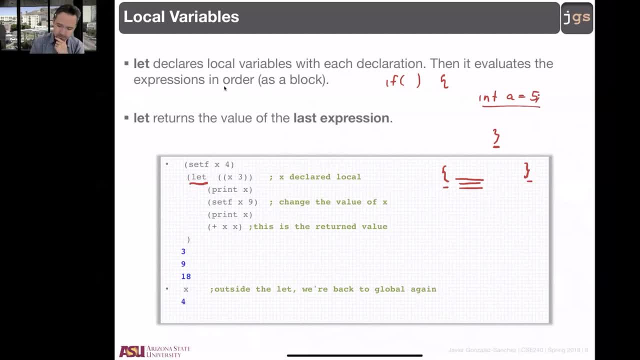 For instance, ZF, X, four. What is happening there? I am creating a variable, a variable, a variable X, and I am storing the value four, That X, local or global, ZF, global. right, It's a global variable. 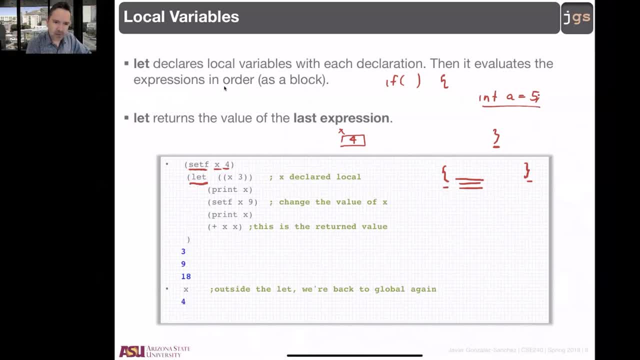 What is the meaning of global? Any instruction in my program is going to be able to use that X. Okay, X global. Then open parentheses let. This is my example. like having this int X equal four global, and surely I am opening curly brackets. 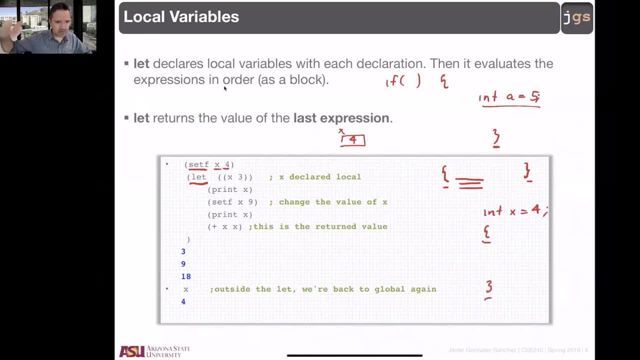 and this can be whatever. again, a method, an if, a for whatever Open curly brackets, let And for the let. what I am going to have is the following: Open parentheses, closing parentheses. The first parameter for let is going to be a list. 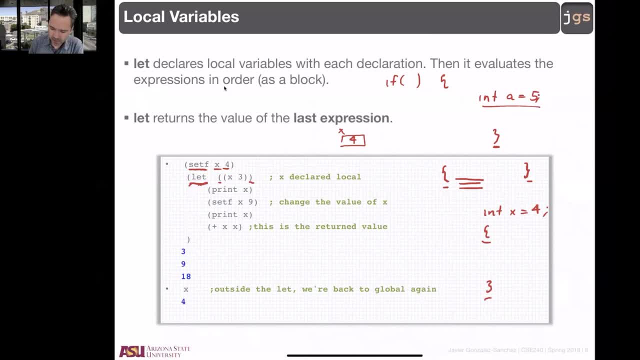 A list of what? Other list? Other list with what? Only two elements? Exactly two elements, Yeah, the name of the variable and the value that you want for that variable. Let parentheses, parentheses X3.. I want out of X local with the value three. 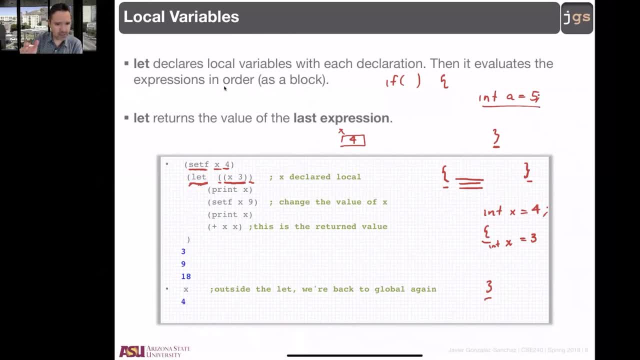 And, as you are going to notice, what I am going to do here is to play with X and that X, from this point to this point, is going to be the X local Because, as you remember, local value, local value, have priority versus global variables. 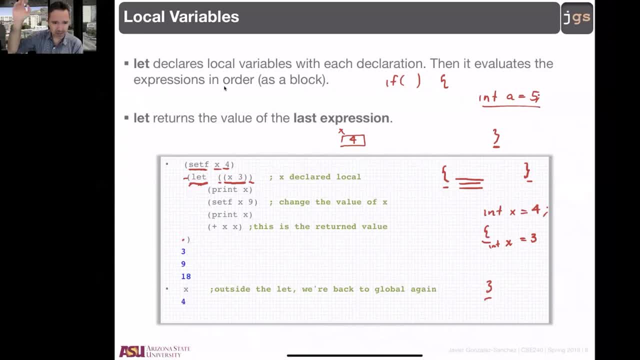 I use my local. if that local have the same name that a global. Can you have more than that? Can you have like: int y equal five, int a equal zero? Yeah, Open parentheses, let open parentheses. and you are telling me that you want x with the value three. 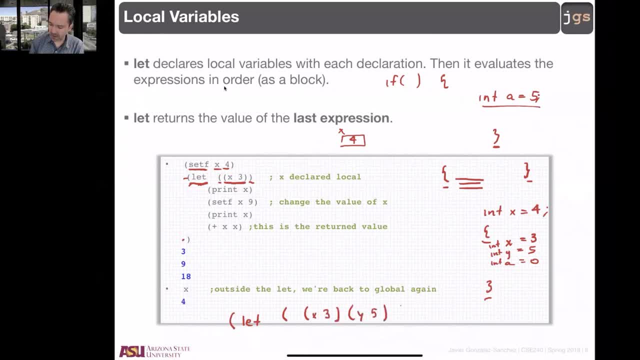 and you are telling me that you want the y with the value five. and you are telling me that you want the a with the value zero. Three variables, good, Done with the variables. Yes, Close the parentheses. These are my local variables altogether. 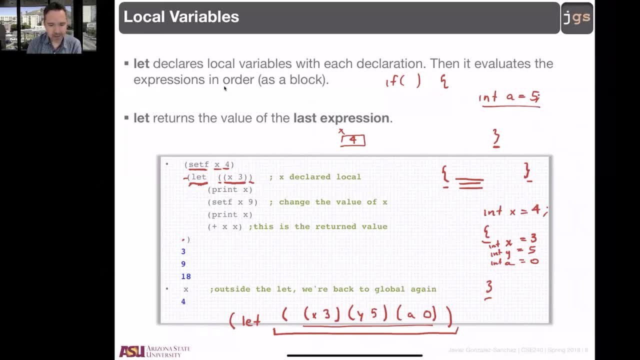 Three local variables. The only thing that I need parentheses name and value. In my example here I only have one, So it looks like parentheses, parentheses, parentheses and another parentheses. It's because inside of the first two 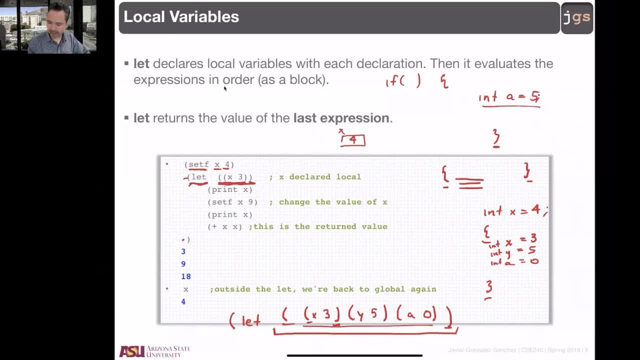 I have all the variables that I want. In that case, one here, three, Okay, what else? This is one parameter, the first parameter, for let all the other parameters and I can have as many as I want- Instructions, instructions such as print set print. 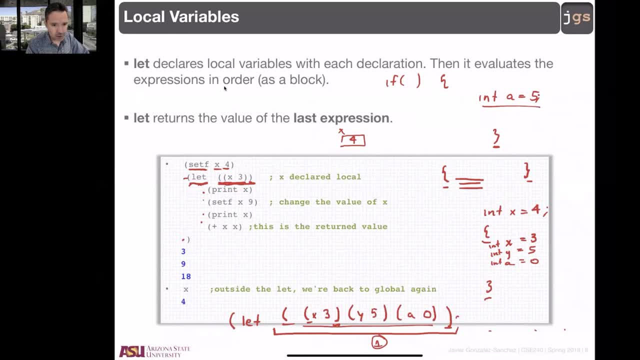 plus and those instructions are going to use all these variables as locals. So if I print x here, hopefully it's clear why I am printing three not four. I have an x here with four and I have another x here with three. 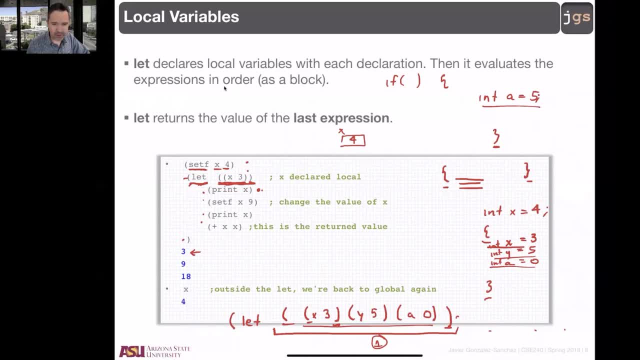 I print x. I print the local, not the global. three: Moving forward, I am going to do a setf. Wait, you told me that setf is to create global variables, but now you are using the setf inside of a let. 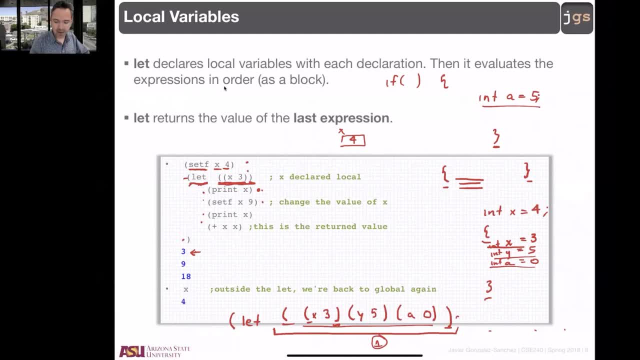 Well, I told you that the setf is equivalent to the equal. If you put a variable equal to some value, that is creating the global variable. but the setf is the equal. So the let is open in a block. Inside of the block. here you create this: x equal three. 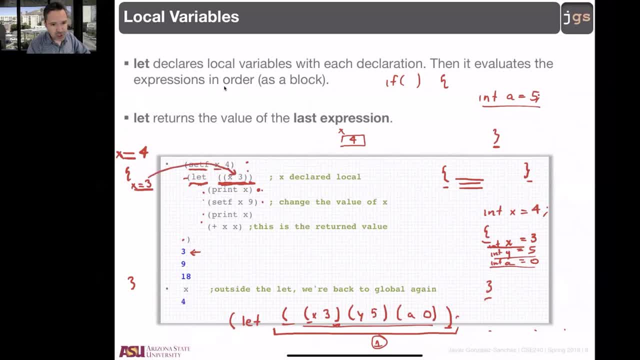 This one is the local. but what happens if you want to change the value for that variable? What happens if you want to do x equal 10 inside of your program? The equal, the equal is the setf. Well, it's a setf and you are using the x. 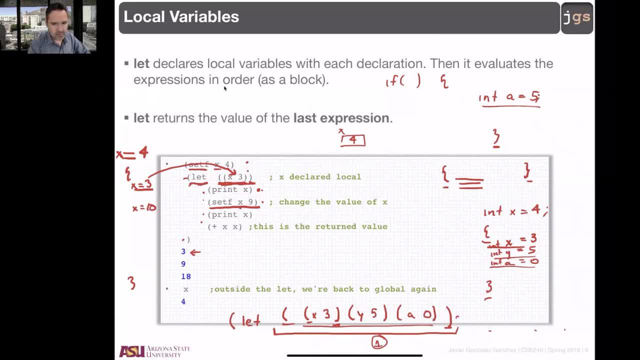 It's going to be the x, local or global, The local, The local, the local have priority. This setf is not creating a new variable because the x already exists. That setf is the equal, the assignation. You are using the setf. 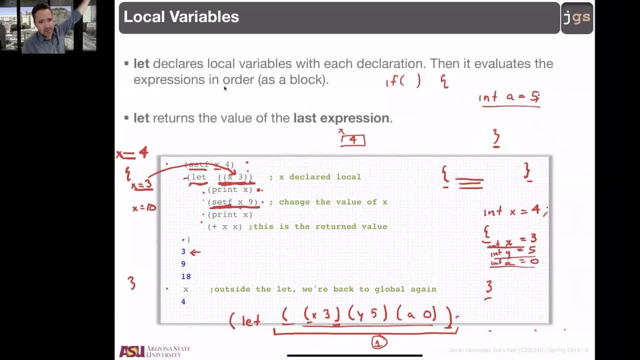 as an assignation And also if the variable do not exist, that setf is creating the variable. Yeah, setf is assignation If you do a setf outside of any other instruction, directly in the common line and that variable in particular. 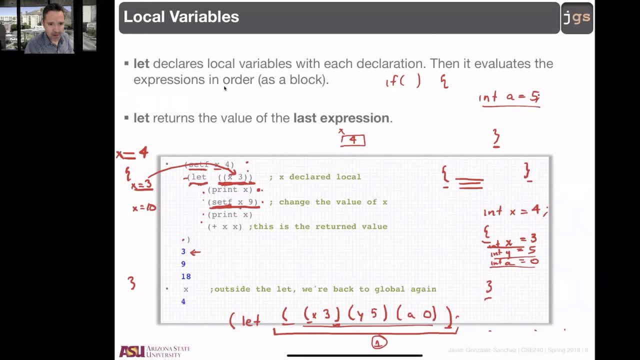 that name do not exist already, it's going to create the variable, like the x before. If the variable already exists, the only thing that is going to happen is I am going to change the value. The same instruction: setf equal. 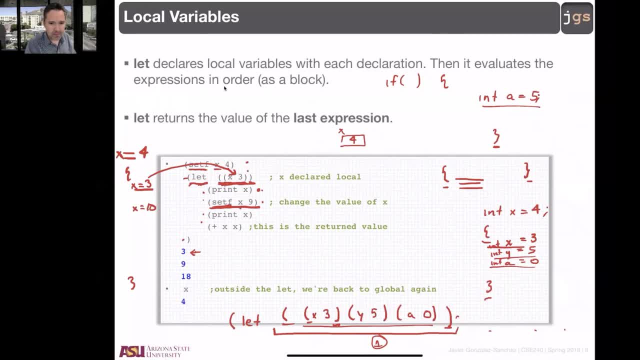 to create a new variable or to change a value. This one is making x equal nine, As I mentioned before, the x local, because I am inside of let And then I am going to print the x, I am going to print the nine. 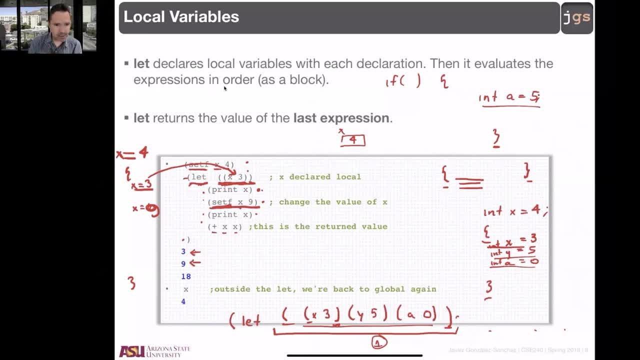 And then I am going to do x plus x, nine Plus nine, And this plus is the last line in the let, Let, in the same way that proc n is going to return the result of the last line And let is going to return that value. 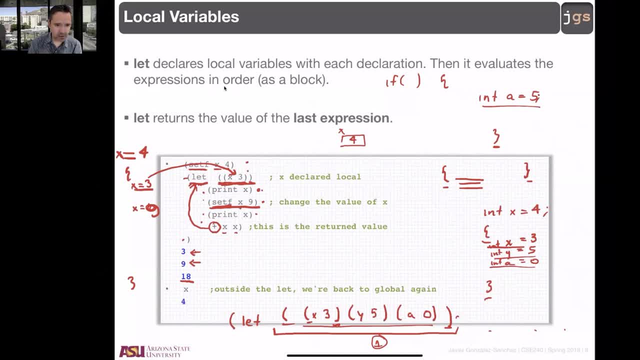 The plus was never printed. The plus was returning to let Let print the result 18.. And if I ask for this x that I mentioned is the same that print x. Notice that this one is outside of the let. I already closed the let here. 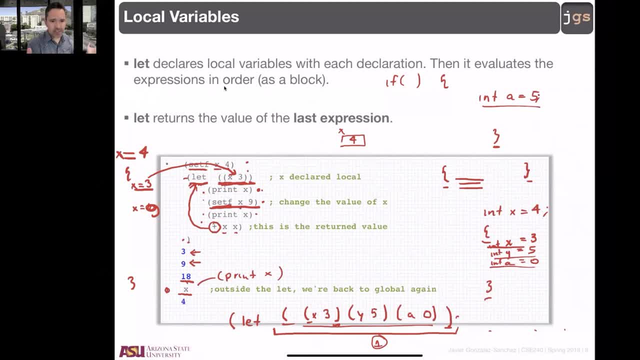 If I ask for a variable x, the local do not exist. We close the let. We close the curly bracket. So all these three nine gone. So all these three nine gone. If I ask for printing x after I close the let. 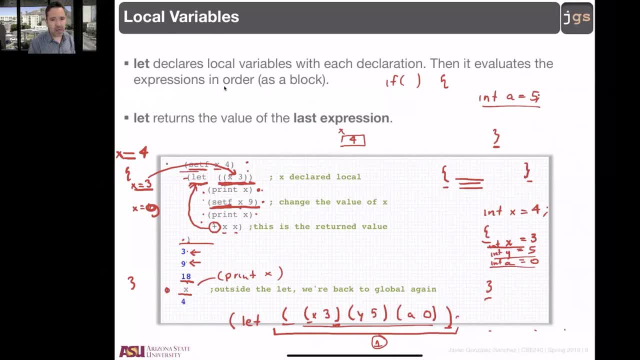 what I already have is my original local variable, that one, And therefore I am going to have a four: Global variables outside of any function, any function, any instruction or any block, proc n or let local variables inside of a block. 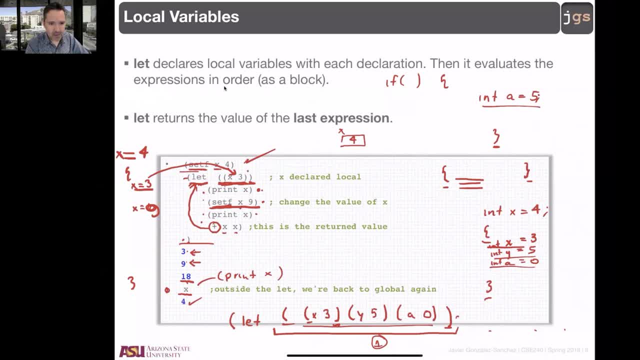 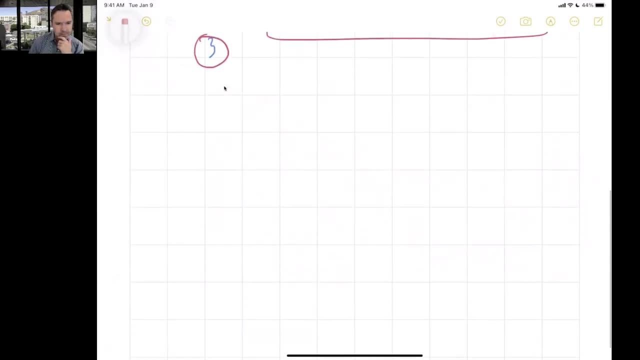 In particular, inside of a block that we create with the instruction let. That's it. Global, local conditions and loops. Okay, so what if I want to do a program in Lisp like for int x? Let's say, I want to create a program in Lisp. 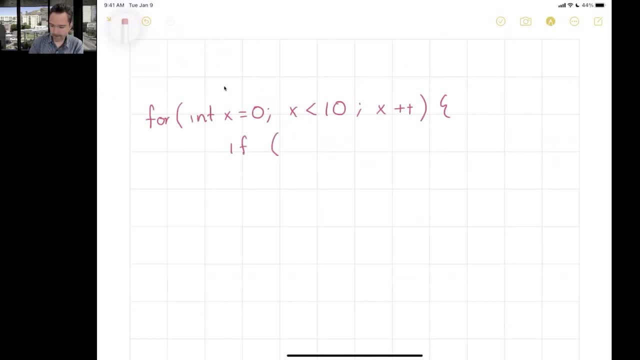 for int x. for int x. You are now going to create that program. What I'm doing now is posting that program into Lisp. It's going to be a four. You can see that now. It's like a four. Thank you. 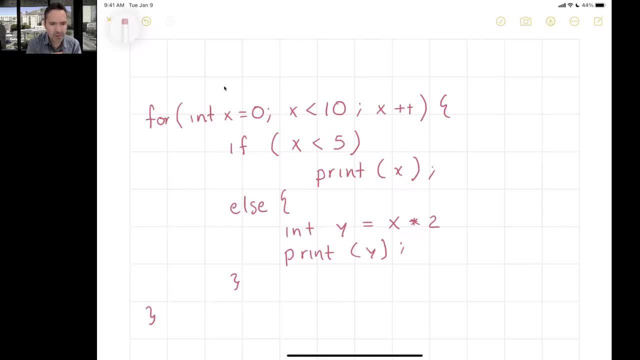 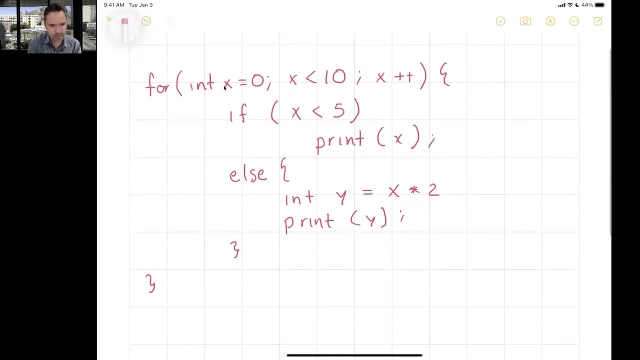 That program? what could be the equivalent of that program in LISP? What instructions do we need? The times If, What are we going to do with these two here? A local variable with an instruction print. It's going to be a PROC N or a LET. 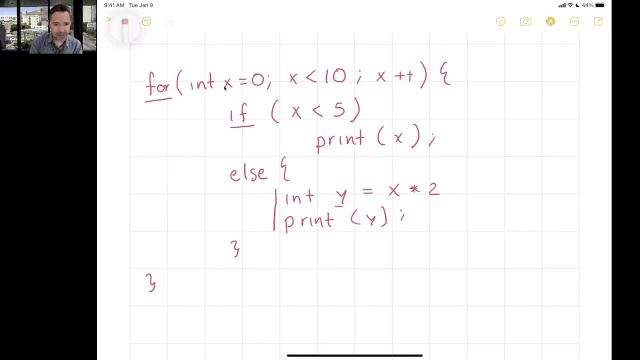 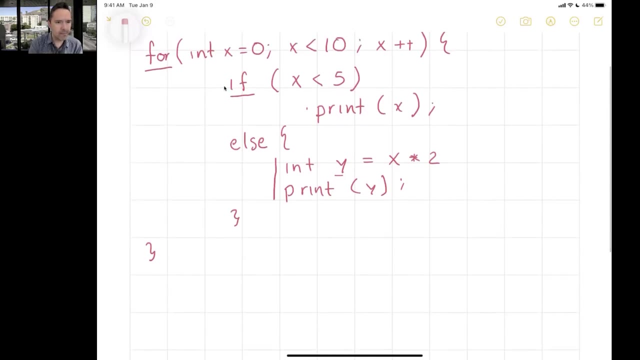 There is a variable here, probably a LET. Do we need a PROC N? Or, in this case, maybe we do not need PROC N? use the LET Here. there is only one instruction: Yes, the doTimes automatically create this variable, used like before, local. 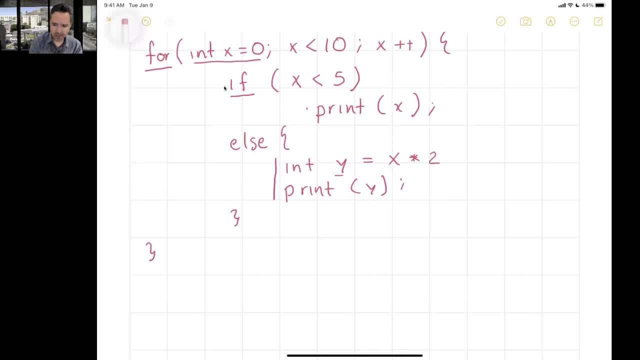 This is a very good example. If you consider this variable X, this variable X do not exist when the for finish is a local variable, a local variable to the loop. So that is the same idea. with the doTime, The variable is going to be local to the loop. 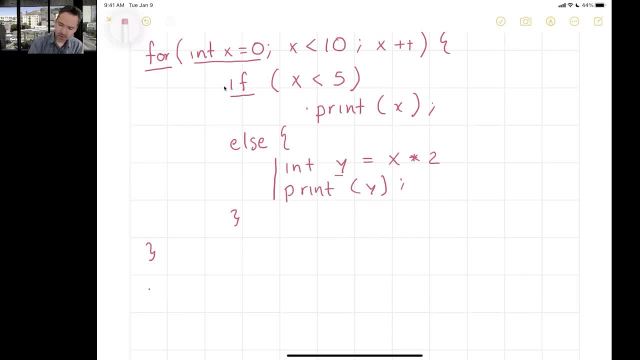 Only exists for the loop For your exam. this is going to be a classical question, a piece of software. and just because now you know the syntax of other languages well, translate. Translate key ideas quickly. Something like that in LISP: 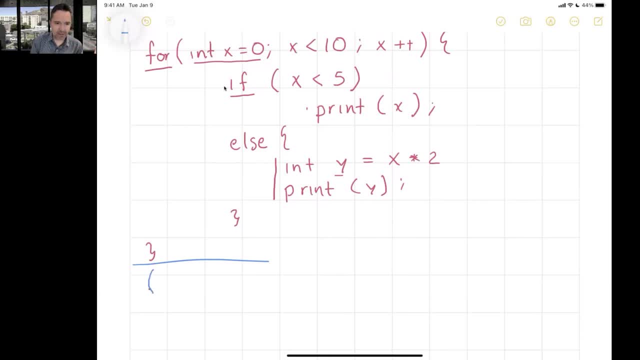 Well, Something is going to start with open parenthesis And the instruction we have for is going to be doTimes, And the next instruction is going to be, again, parenthesis, And something that you need to remember is: well, what is the first parameter of doTimes? 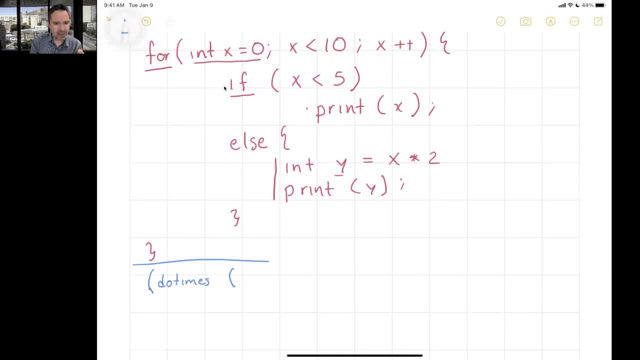 For the first time, we use something here that is not an instruction. For the first time, whatever is here, It is not an instruction, It is not going to be executed, It is just a collection of data. right, The variable. 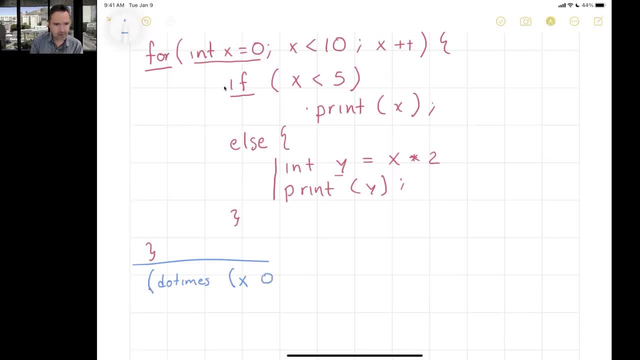 Then The number of times. Then I can ignore the return. but if you want to return something it should be there. Yeah, Remember the idea. here is where this number is how many times the loop is going to rule. So you can imagine: equal to zero, lower than 10 is going to be 10 times zero to nine. or if you want to imagine one, two lower or equal to 10 is going to be 10 times. so the number is how many times the loop is going to rule, not exactly the lower than something. 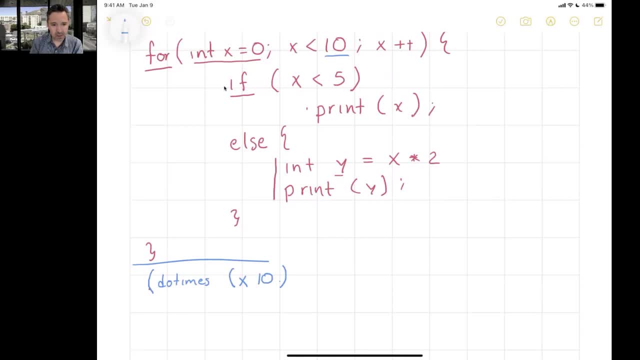 or if you think complex, it is too easy to lose some control. If you think about lower than something, start with zero And that's it. Anyway, do time, And then we can start with the instructions. Remember, do time, and then we can start with the instructions. 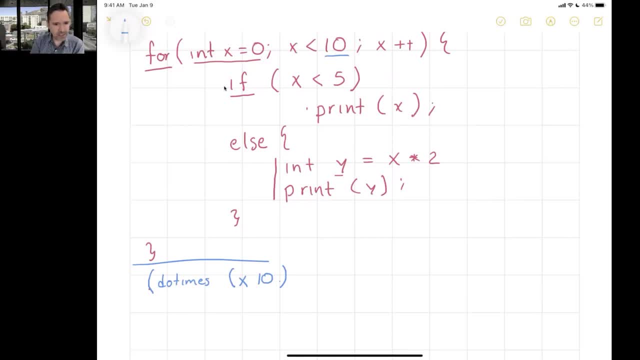 Right Everything after this small configuration thing. it is the instructions. And well, the instructions Open parenthesis, And I already started with the if Not. this is also useful because you can use tabs Like before, enters Like before. 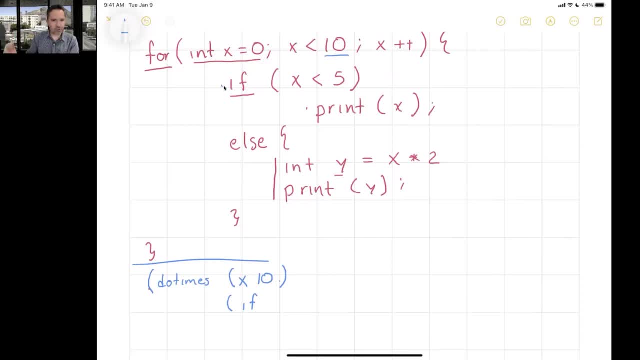 You can also for older Schul durum, then you could start with. if lessonsfollow for next set of tasks, Like for older Schul durum, so you can start with if lessonsfollow for next set of tasks, can use whatever you need in order to structure your program, as always for the computer. 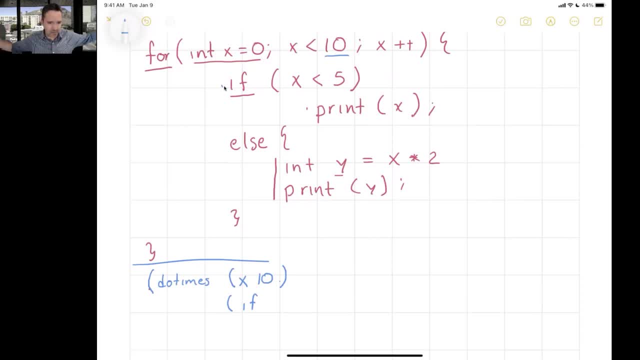 All those things the computer don't care For. the computer you can write a big line and it's fine. It's a bad idea: You can get lost, So taps enters. it's a good idea to structure things: If, the condition, parentheses After the condition, the if body and the else. 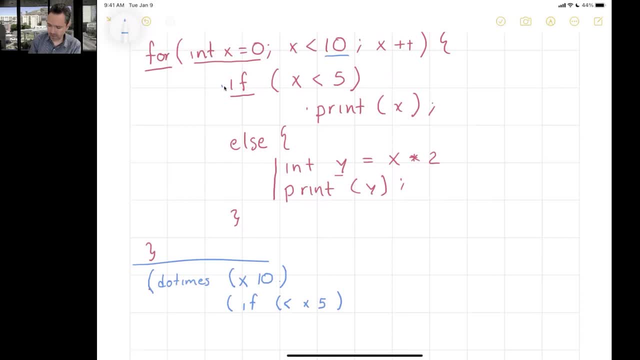 body. the if body is pretty simple: Parentheses, the instruction, the parameters, Okay, And then the else part. For the else, what I have is this: curly brackets. because I need a body For the curly brackets. I have two options: Proc n or let. In particular this: 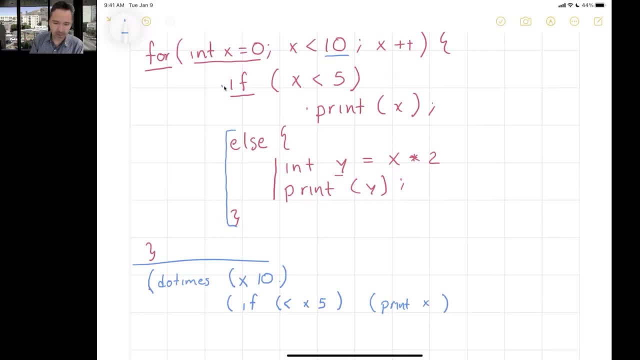 one is asking me for a let because there is a variable. let, Allow me to create variables. So for the let, Okay, I do not need the bracket or the else, I'll use this space and the next instruction correspond to the else Let for the let. important to remember parentheses. Inside of these parentheses: 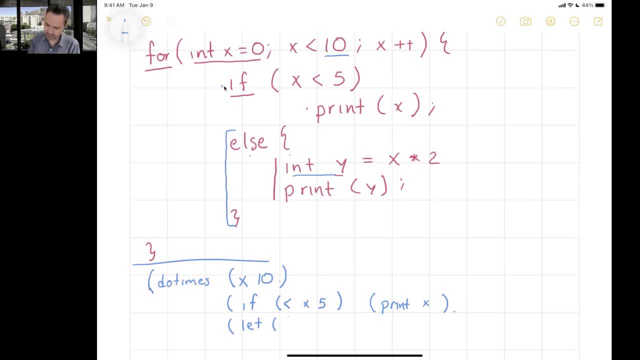 are going to be all the variables Here. I want a variable y. I want an initial value for that variable y. That initial value is going to be a multiplication. This is my variable y. I can create more variables here. I do not want more, I only have the need for. 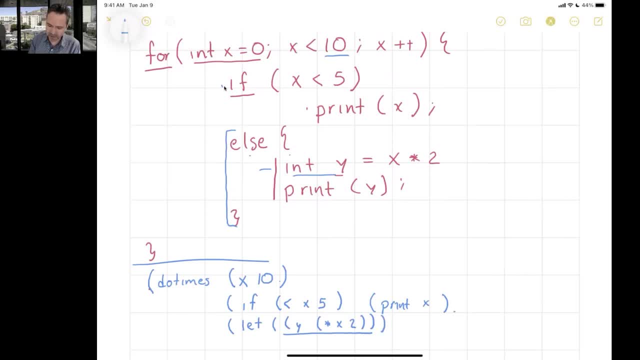 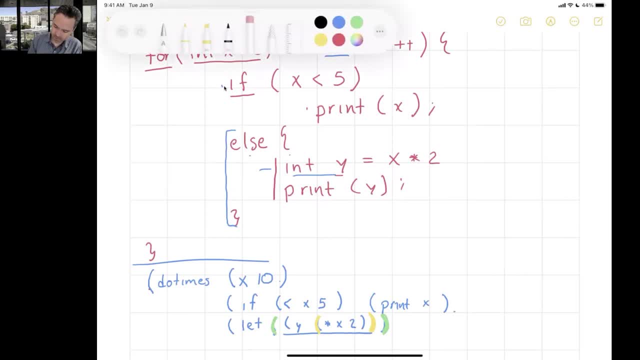 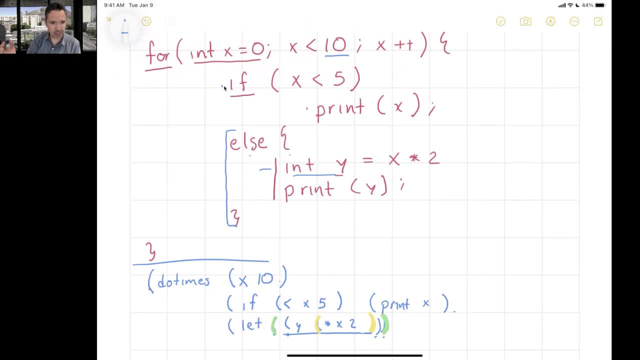 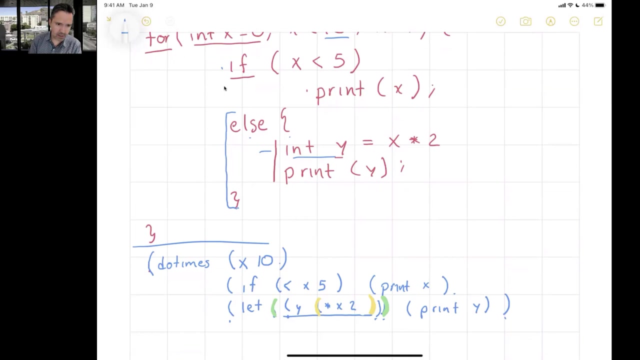 And after that I can put the instructions that are inside of the let. It's a print- And finally, I can close the let, and when I close the let, I am closing this body there. The last thing that I need to do is to close the loop, and I can put this parenthesis here: 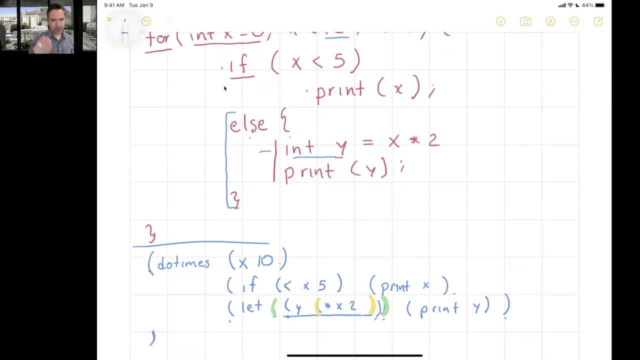 so match with the opening and somehow in red, one program with four ifs in a different syntactical way With other languages and my equivalence with Lisp. any question, The X is literally a variable and therefore have values, and each time that the loop run,